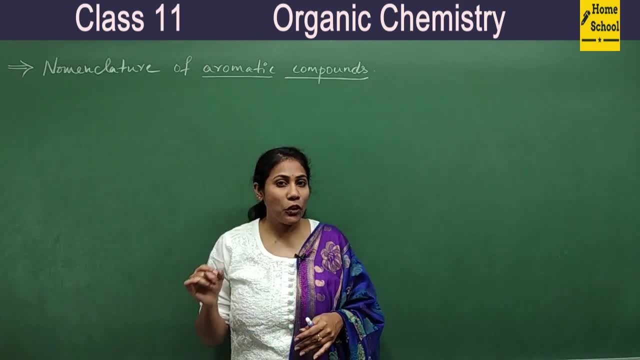 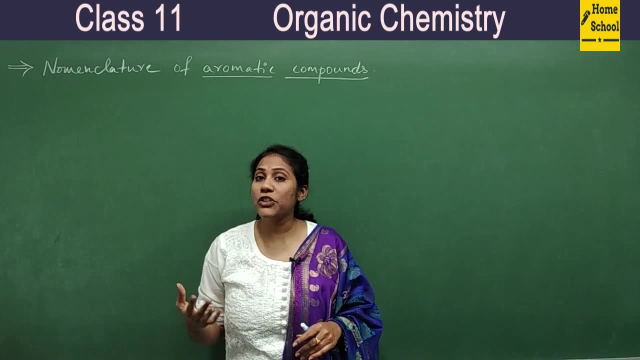 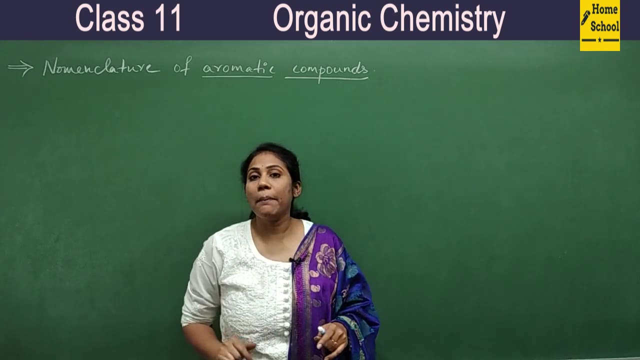 Later in my next video, I have taught you nomenclature of unsaturated hydrocarbons. Later we discussed about nomenclature of organic compounds with functional group, And in my previous video I taught everything about how to name alicyclic compounds. And now 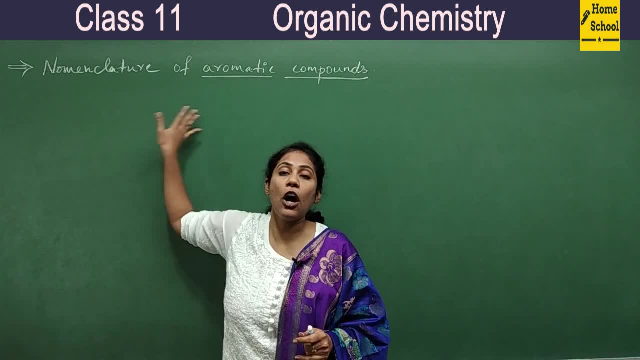 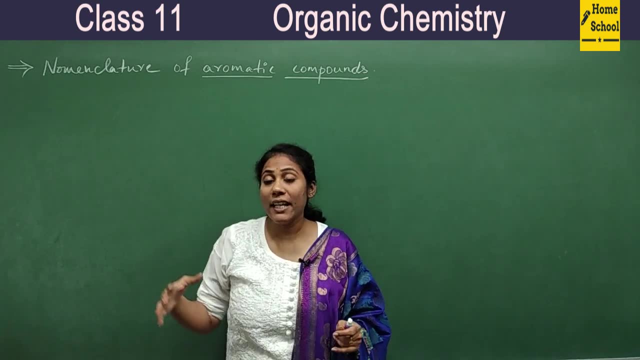 we will discuss about nomenclature of aromatic compounds. So we know what do we mean by nomenclature of aromatic compounds. So we know what do we mean by nomenclature of aromatic compounds, Isn't it? Benzene and benzene-like compounds are called aromatic. 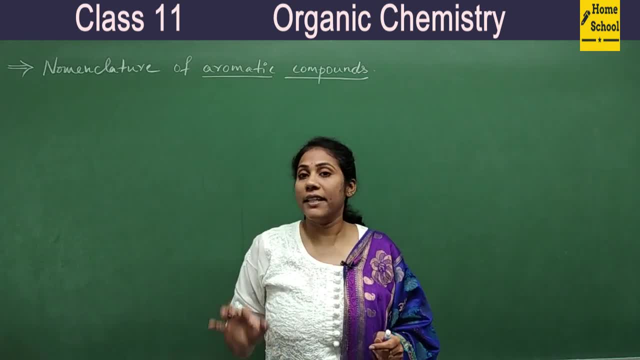 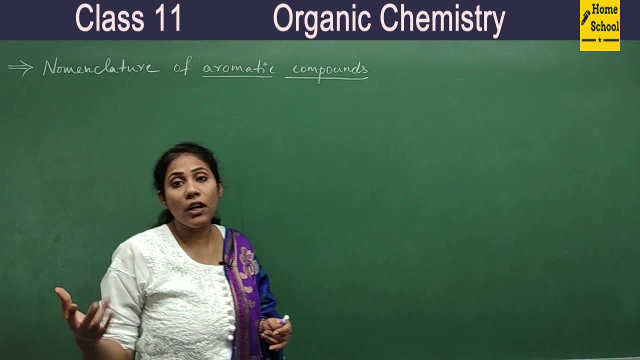 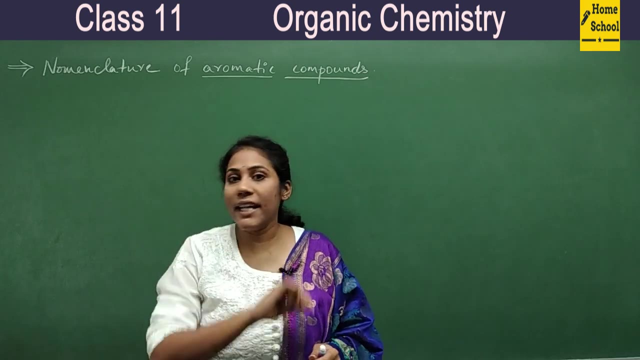 compounds. Why we call them as aromatic is because they have a special smell. They have a peculiar smell, So we call them aromatic compounds And there are many conditions that they have to satisfy to be called as aromatic compounds, And all those conditions we will. 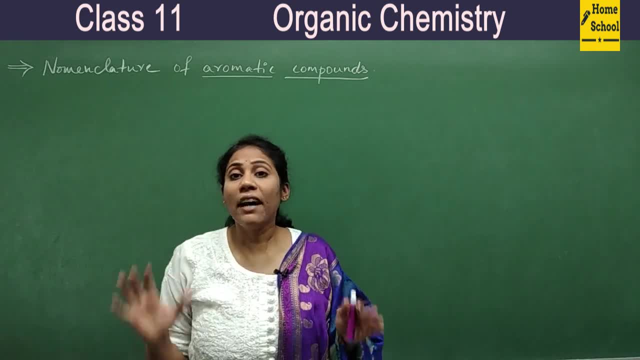 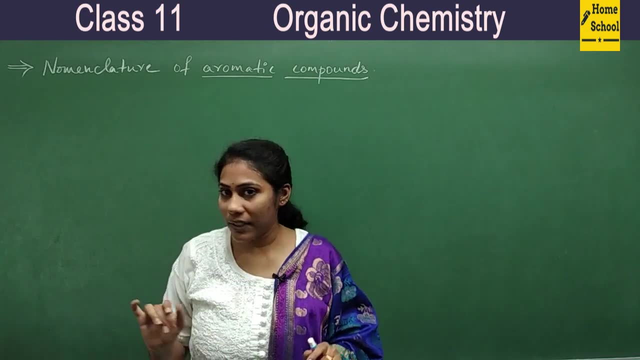 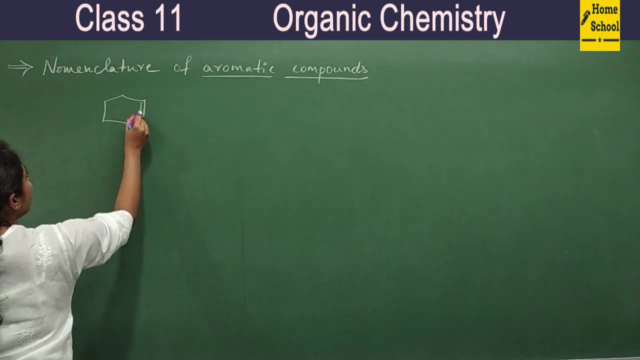 study in our next chapter. Fine, Now we will concentrate only about naming of benzene-benzene-related compounds. Clear, Fine. And the moment I say benzene, then quickly you will write the structure this Right. So its formula is C6H6.. So this is called as benzene. Common name is benzene. IUPAC name is: 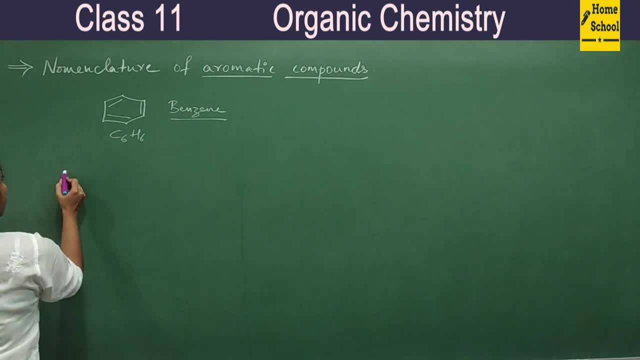 also benzene, And now we will study some of monosubstituted benzene. Ok, Mono substituted benzene, That means if any one of the hydrogen is replaced by any group, then how to name it? You know what? Here there are like six carbons, and in each and every carbon you have hydrogen. 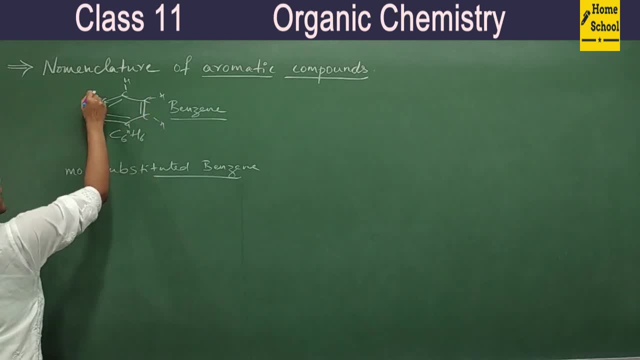 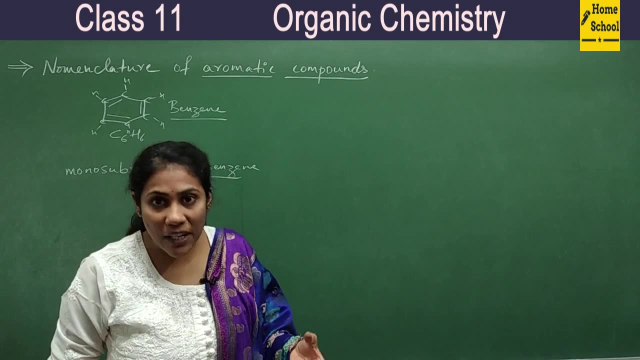 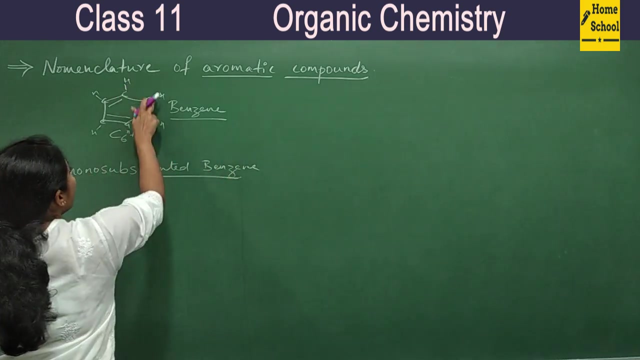 isnt a Fine. Ok, So then what will you name each one of them? Now let's let's like, calculate as many. any one of the hydrogen is substituted by other groups. it can be a substituent group, it can be a functional group, right? so if you have some other groups instead of any one of the hydrogen, then 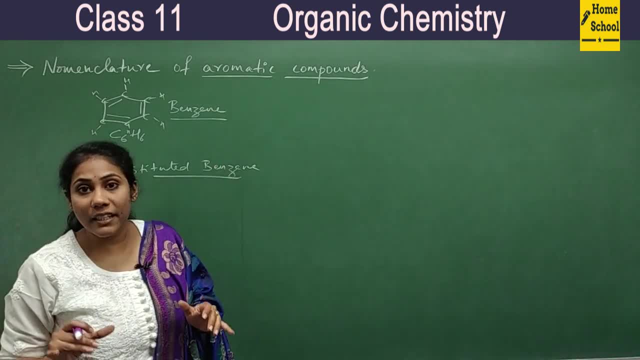 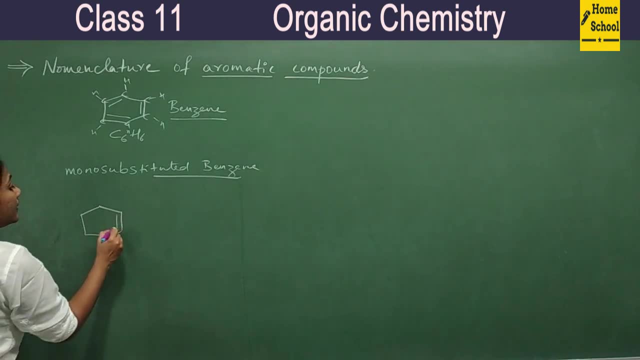 they are called as mono substituted benzene compounds. so let us first study how to give names for those compounds. the very, very important compound that we come across in our study is this: here, one of the hydrogen at this carbon is substituted by methyl group. so how do you? 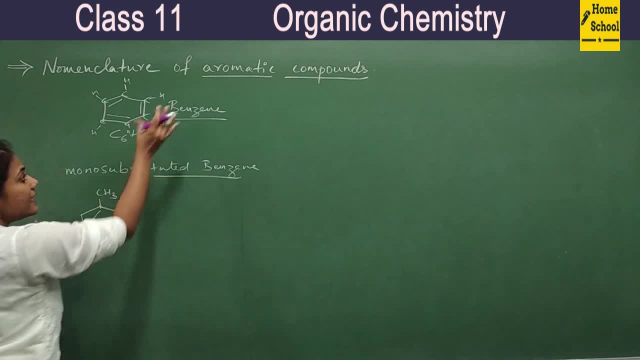 name. this particular compound, benzene, is the code name. benzene should be as word root, okay, and this is like a branch and this is actually a substituent group. then it is actually a compound and its name should be there as prefix. you have to write its name as: 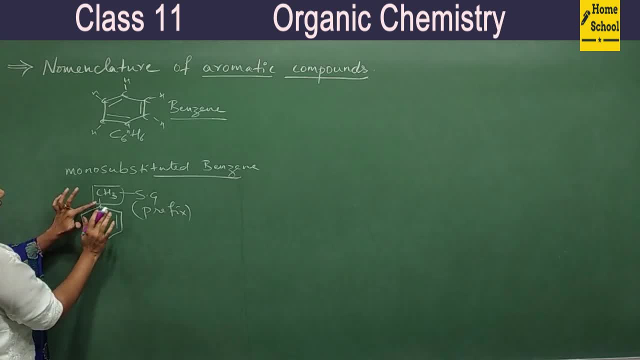 prefix. so what can be its name? its name is one: methyl. so wherever this group is there, that particular carbon gets number one position. remember this. so this compound can be named as one methyl benzene. right, okay, some common name. We call this compound as toluene, Some pronounce it as toluene, So anything. 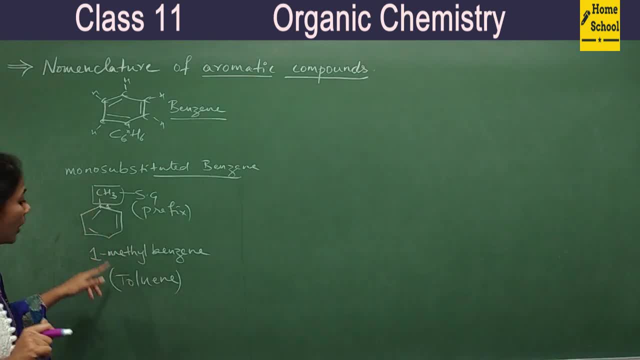 is fine. So this is toluene, And toluene is the widely accepted IUPAC name. Okay, So you can call it as one methyl benzene, or you can call it as toluene also, So toluene is like common name as. 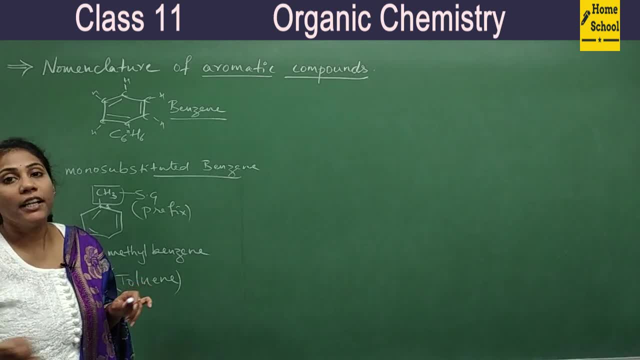 well as it was accepted as IUPAC name. Okay, So this is our toluene. First important monosubstituted benzene. Monosubstituted, That means if single substituent group is there, then monosubstituted. 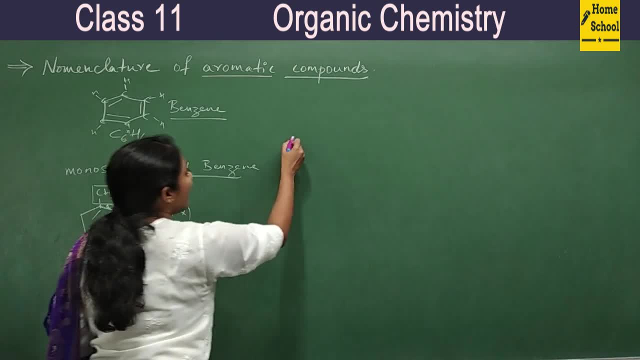 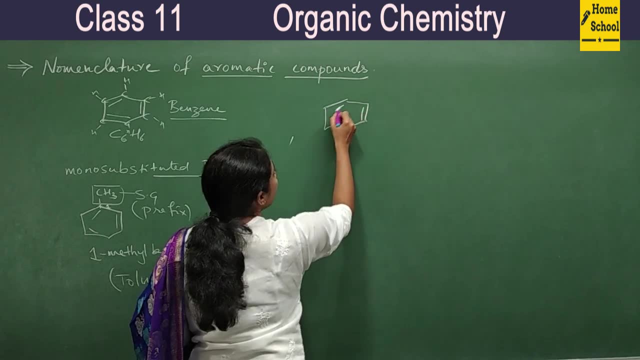 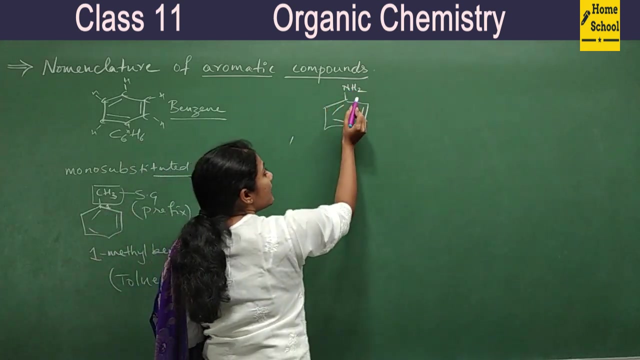 benzene, we say Okay, Fine. And now, coming back to another example for monosubstituted benzene, Observe here: This is also very, very important compound, So I will have NH2.. So here NH2 is like branch which is present at first carbon And its name. 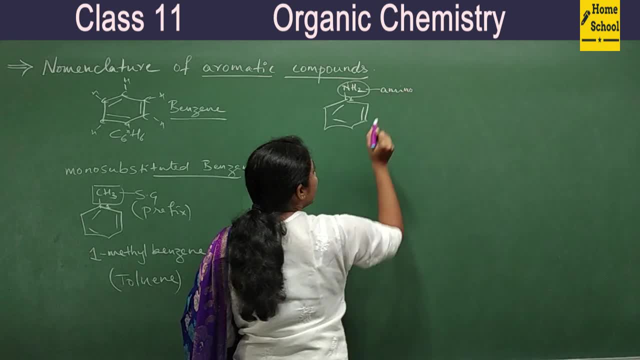 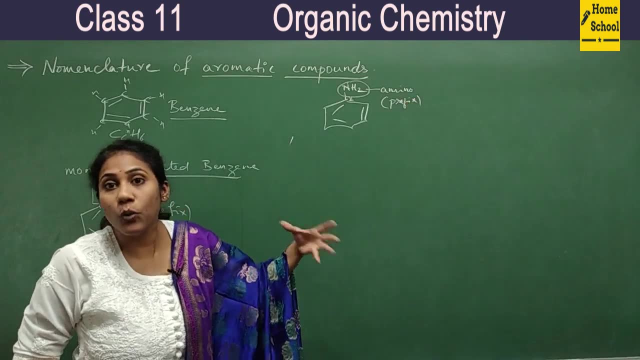 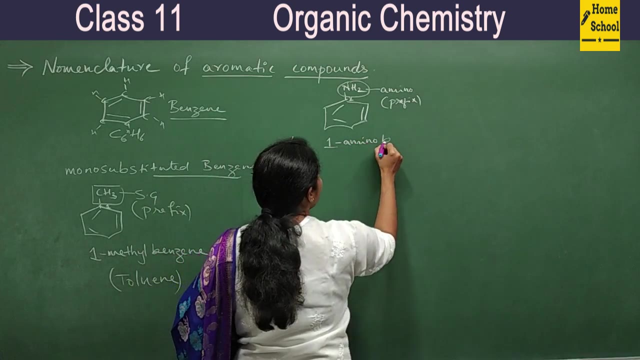 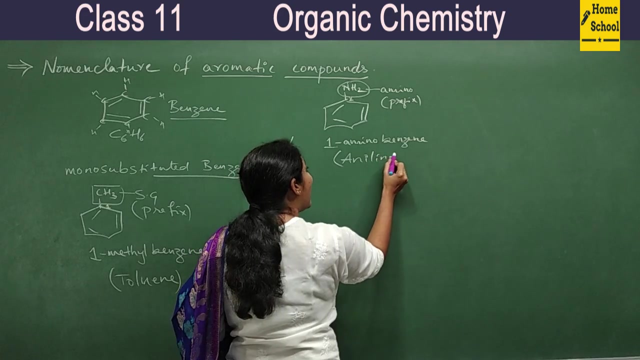 is amino, You will write its name as amino as prefix. Okay, So you will indicate its name. I mean amino in the form of prefix. So we write it as one amino benzene, One amino benzene, And it has a common name, widely accepted name, that is aniline. So very, very important to 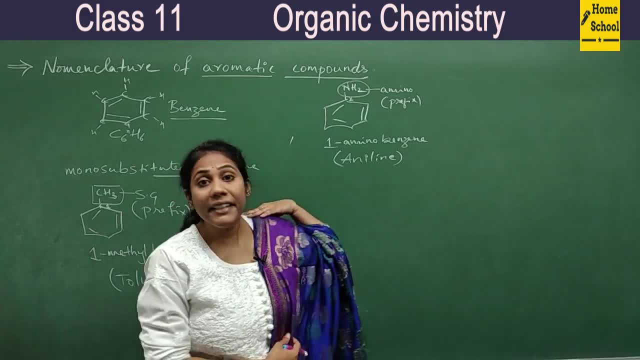 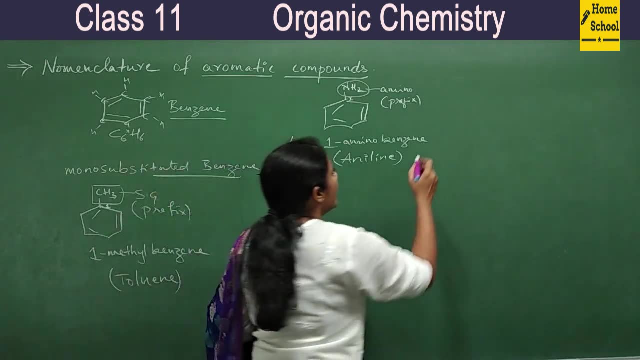 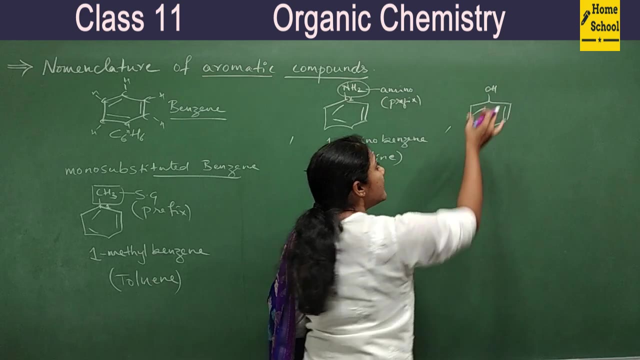 remember these common names. Actually, aniline is widely accepted IUPAC name for this particular compound. Okay, Fine, And the next compound very, very important is this one: And now, this is like a functional group. OH is a functional group, Alcoholic group, Isn't it? So this is a. 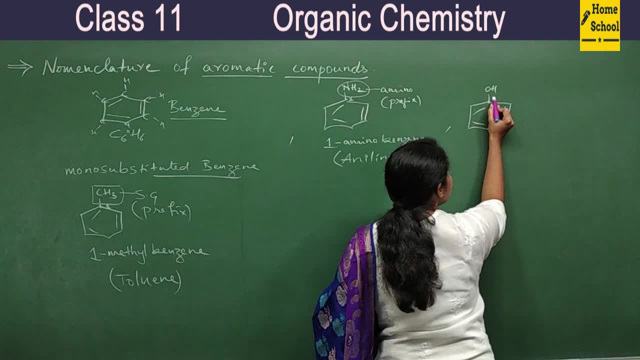 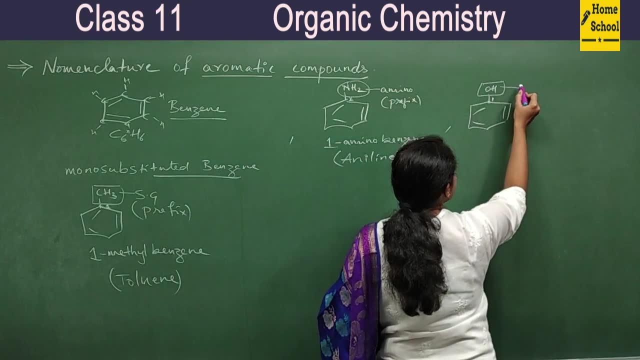 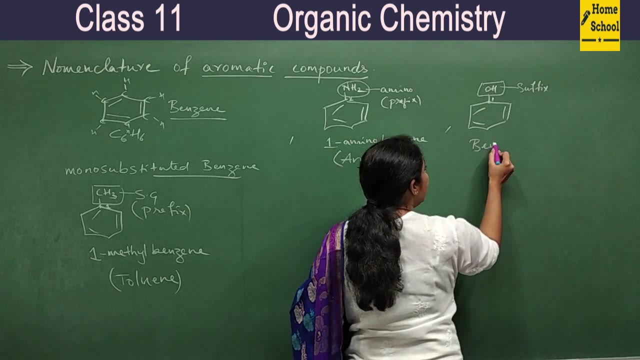 functional group And it is present at this carbon, And this carbon gets number one position. And now, whenever a functional group is there and you know its name, you will mention as suffix, Right? So how do you name this? Benzene? Benzene One All, Or we can also call it as: 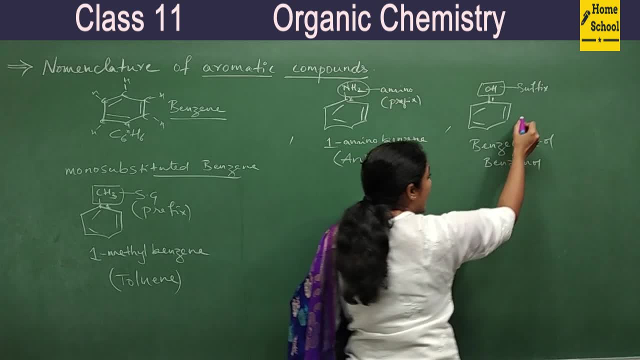 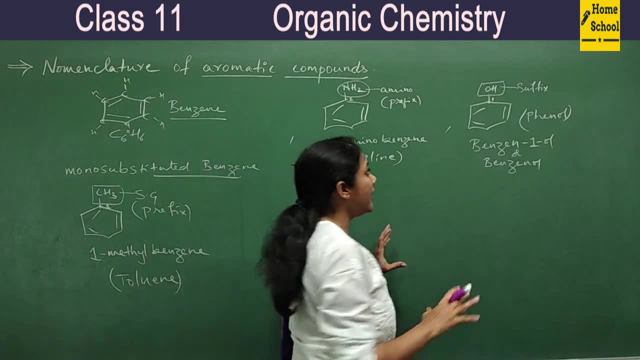 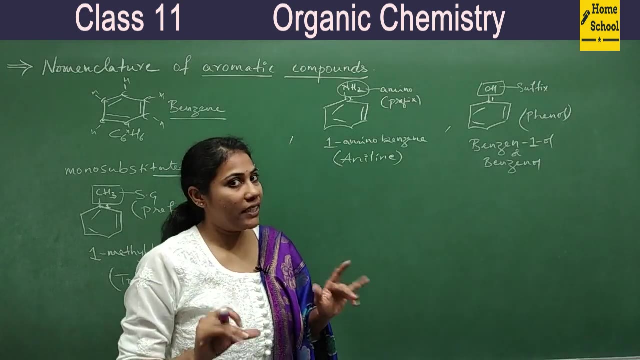 benzinol And it has got a common name. We call this compound as benzinol And it has got a common compound with the name phenol. Okay, So very, very important. Actually, phenol is widely accepted IUPAC name also. So phenol, Very, very important compound. So the next compound, mono substituted: 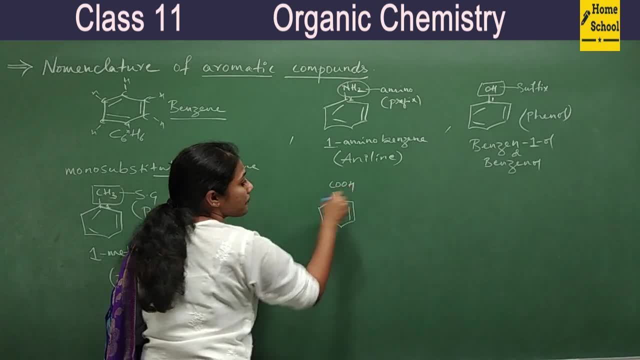 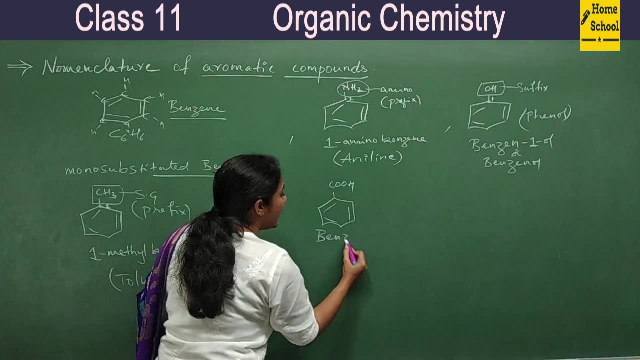 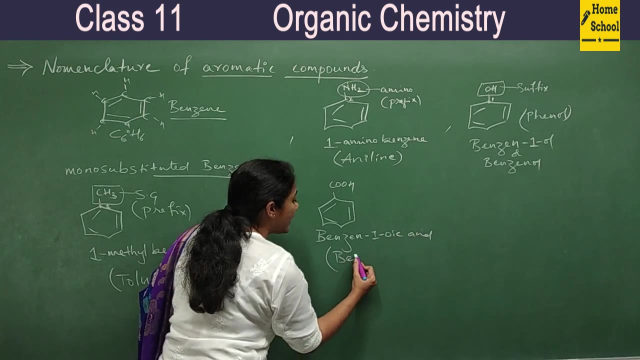 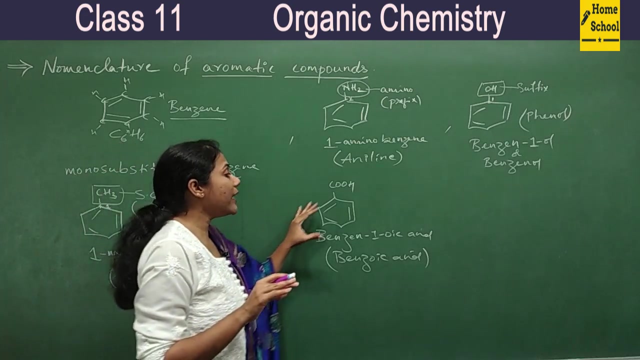 benzene itself. You see this Right. So what may be its name? Benzene One O Greek acid. You can call it as benzene One O O acid, or this is also called with the name benzoic acid, benzoic acid, okay, or you can also call this. 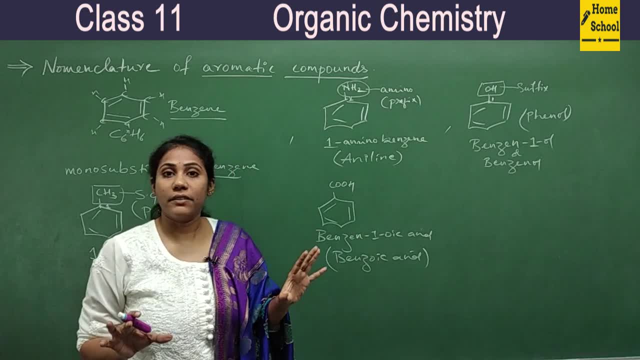 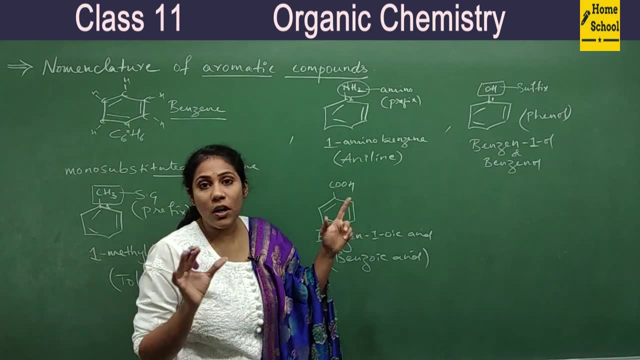 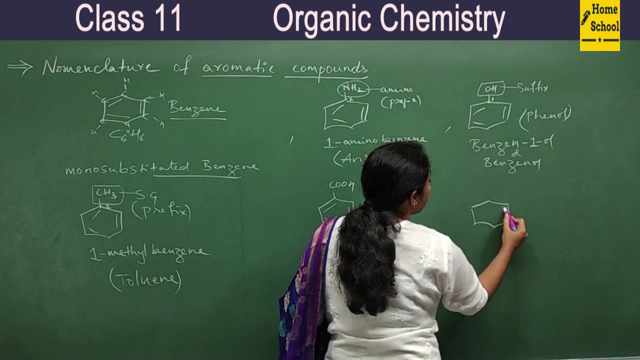 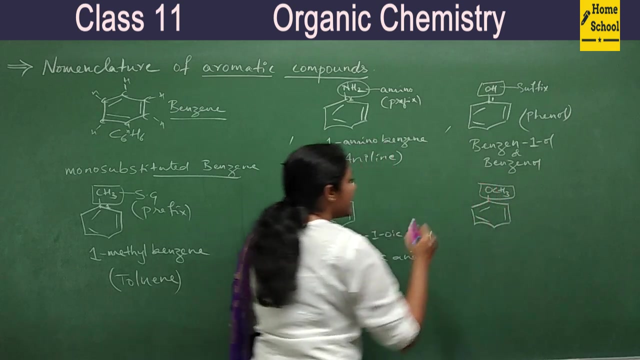 as benzene carboxylic acid. okay, so that is a new way of naming this particular compound. it is benzene carboxylic acid. that way also you can call fine. so the next compound, very, very important- is OCH3. okay, and this OCH3 is different. CH3 is different. okay, and even this is considered. 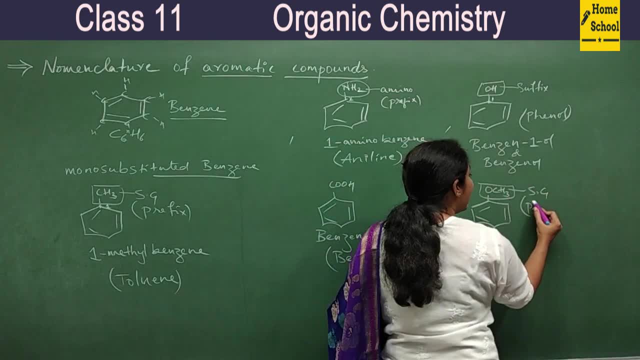 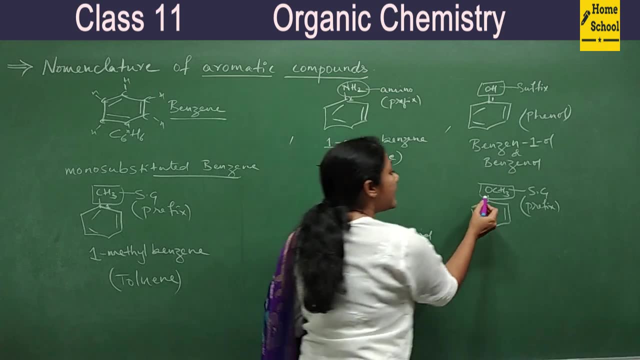 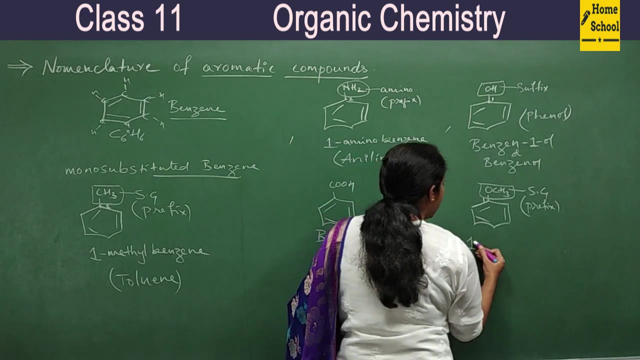 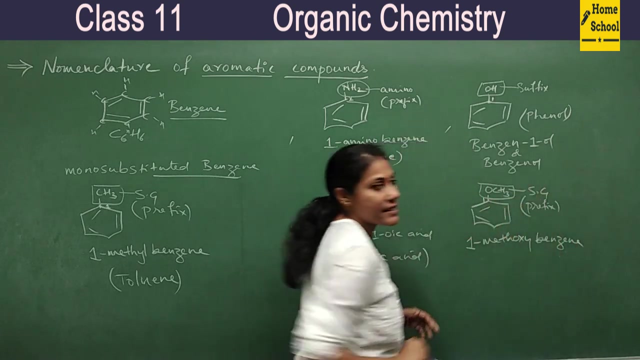 as a substituent group and its name is written as prefix clear and its name is methoxy. so this methoxy group is present at this carbon, so that carbon gets number one position. so so I can call this as one methoxy benzene. so this is methoxy benzene and commonly this is called. 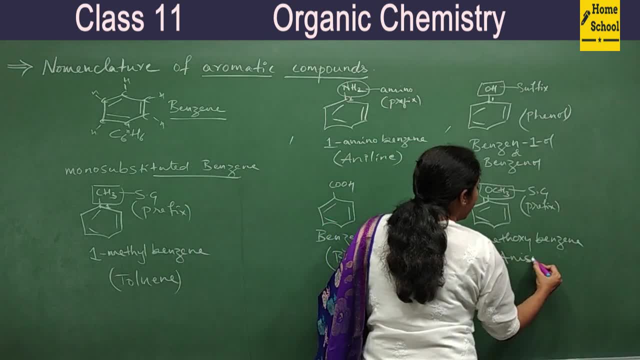 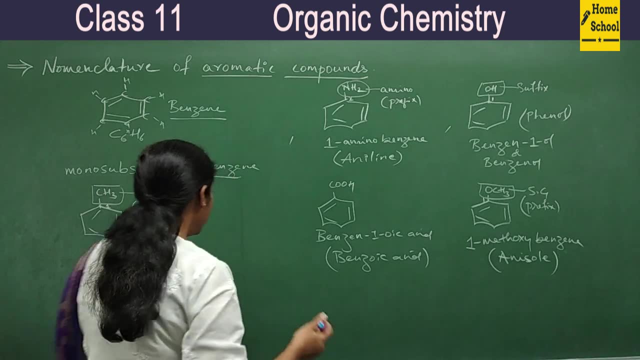 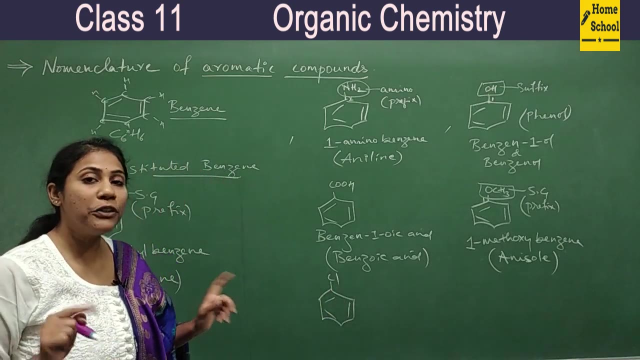 with the name anisole. this is called with the name anisole clear. so all these are very, very important compounds. and let me give you some other compounds. see here, chlorine is there, so how do you name it as chlorine? and similarly, we have that. this is now. this is one chloratre lor benzene, one cloro benzene. so this: 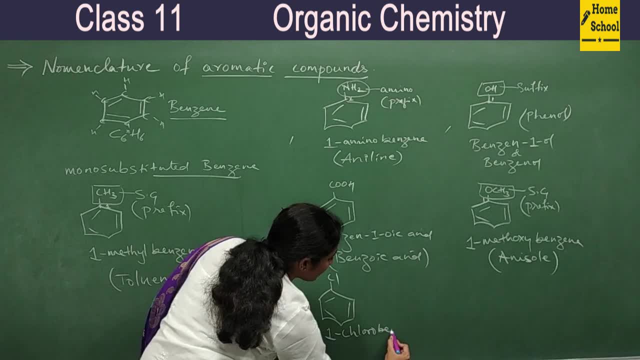 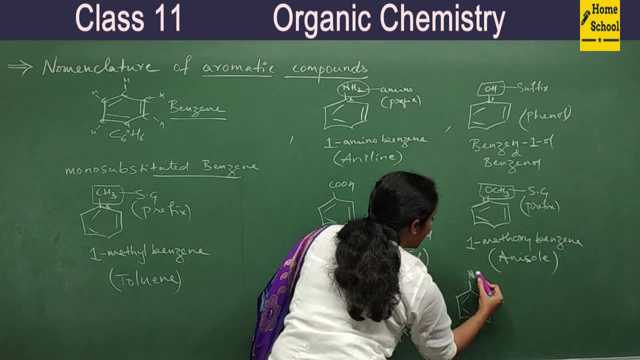 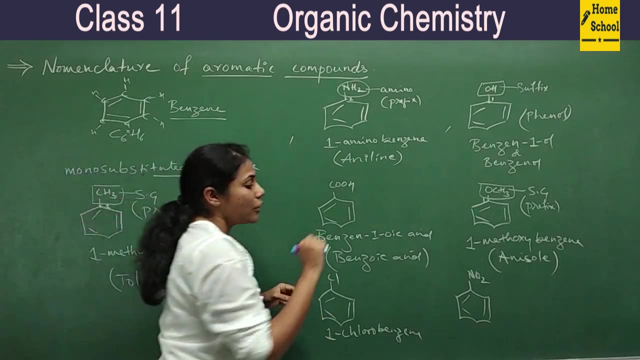 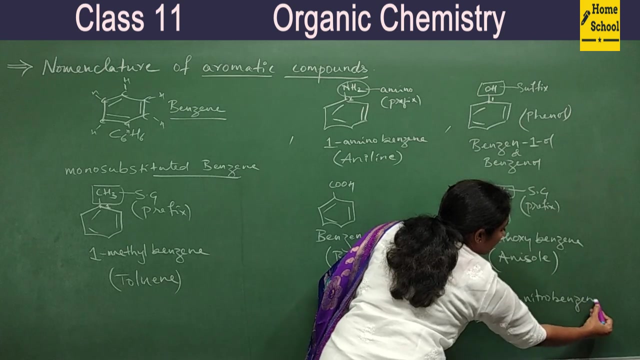 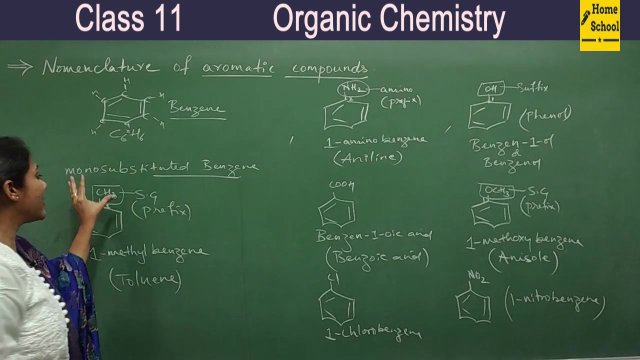 is one chloro benzene, and similarly this is also very famous compound, enjardin. so nitro group is like a substituent group. its name is written as a prefix, so you can call this compound as one nitro. this is how monosubstituted benzenes can be named. So if you have a single substituent group, 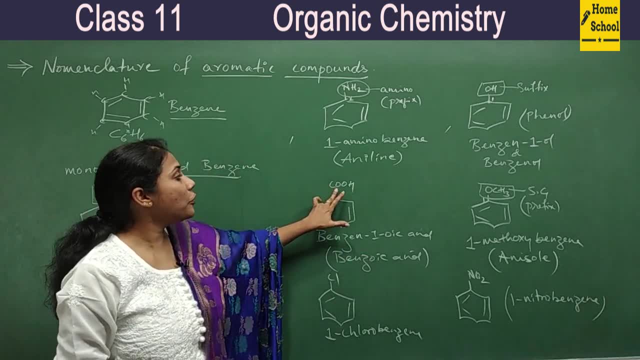 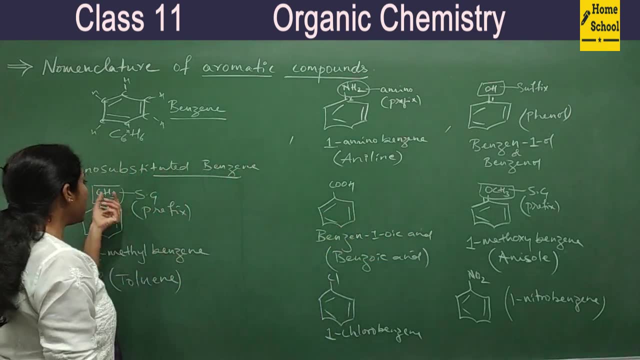 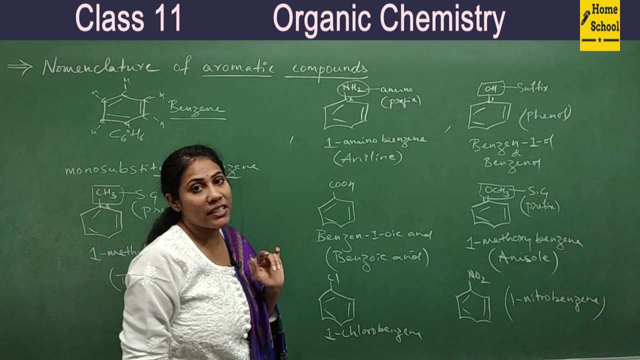 or single functional group. if it is a functional group, like COOHOH, their names will come as suffix. If it is like substituent groups like CH3, OCH3, NO2CL, you know their names will come in the form of prefix, right? Fine, So now we will go for naming disubstituted benzene. 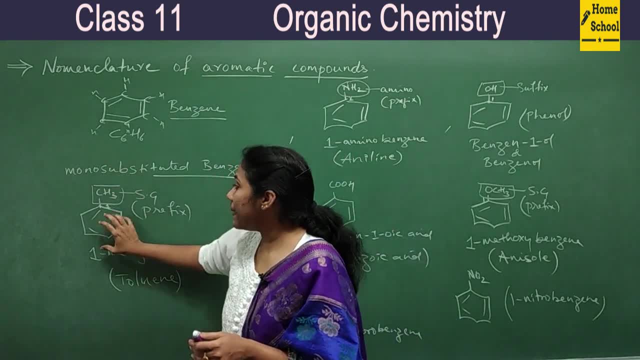 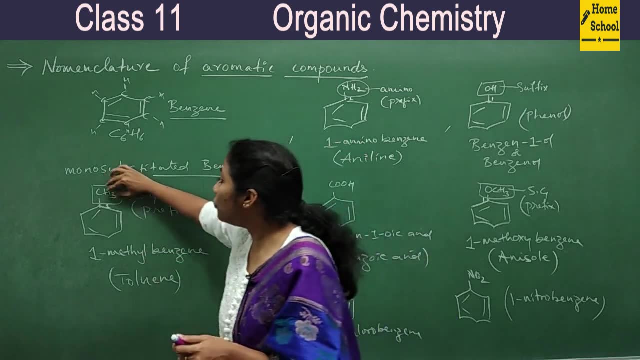 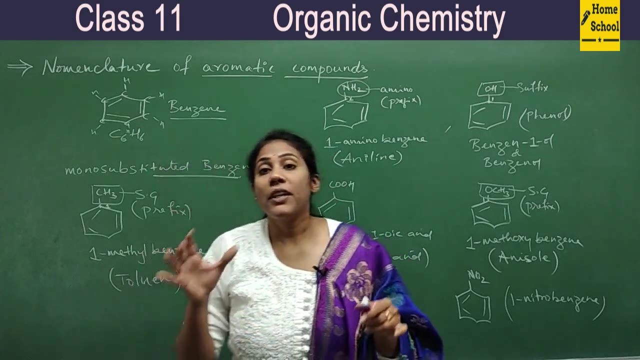 I mean if you have two such groups in a benzene, if another hydrogen also replaced by another group, right? So if you have two substituent groups on this benzene ring, then we call it as disubstituted benzene. So let us discuss the naming of such compounds First. you observe: 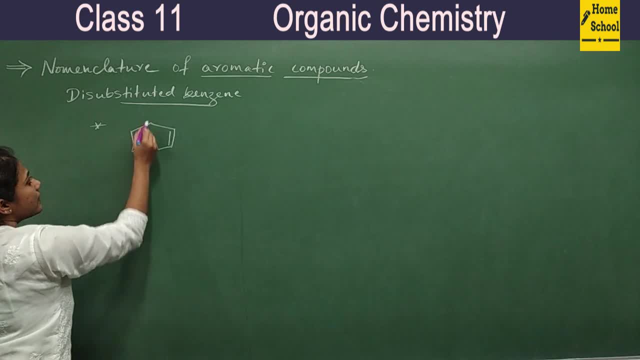 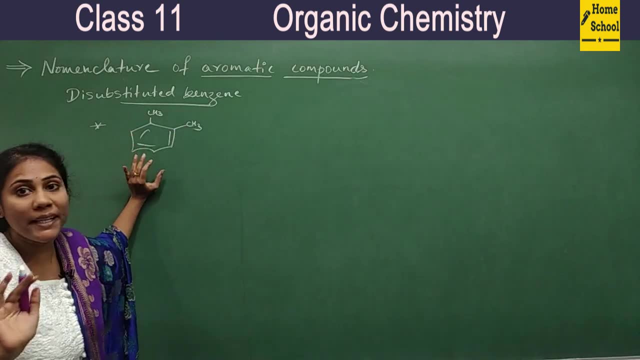 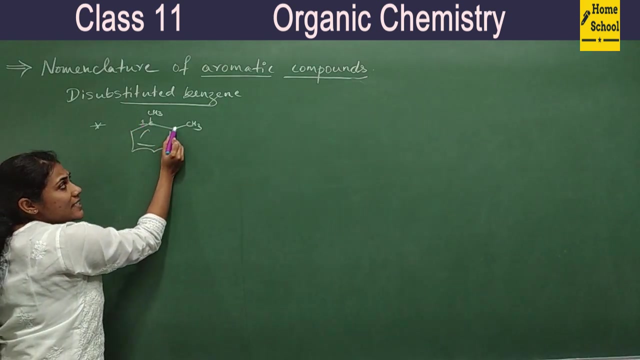 this compound. You see this, There is one methyl group and another methyl group at this position, So two methyl groups are present on benzene ring. So how you can name this? Consider this carbon as number 1 or you can consider this as number 1.. Okay, If you consider. 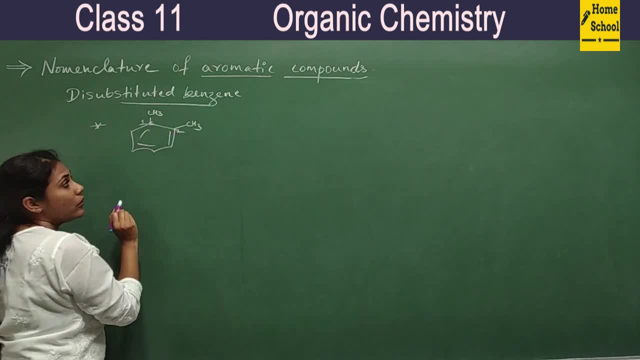 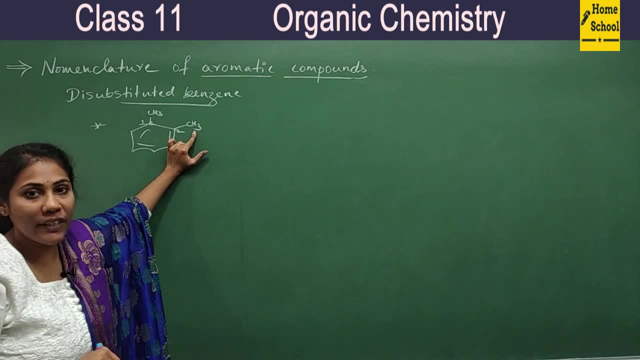 this carbon as number 1 and this must be 2.. Okay, So the next numbering should be on a carbon atom which has got next numbering. So next numbering should be on a carbon atom which has got next substituent group. Okay, So you cannot go in numbering this way, You should. 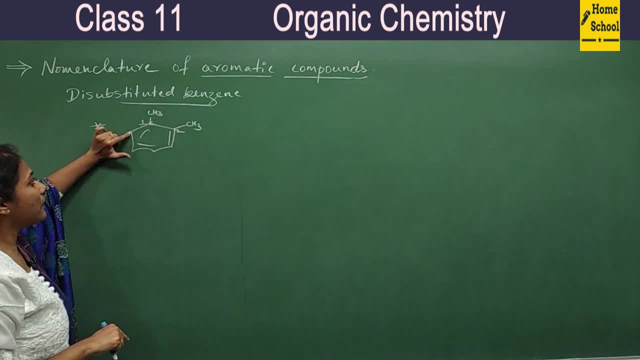 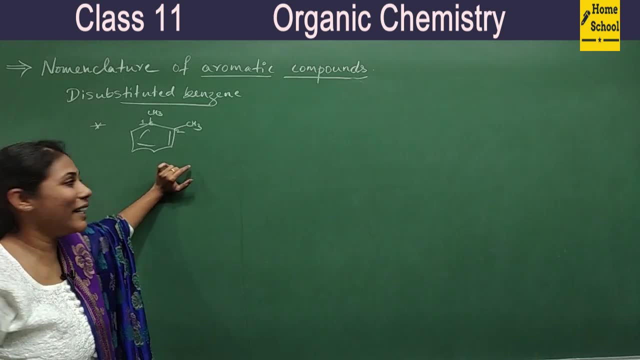 go numbering this way right. So if you number this as carbon 2, it is waste. I mean, this gets number 6.. You must actually follow the lowest locant rule here also. Okay, So number 1,. 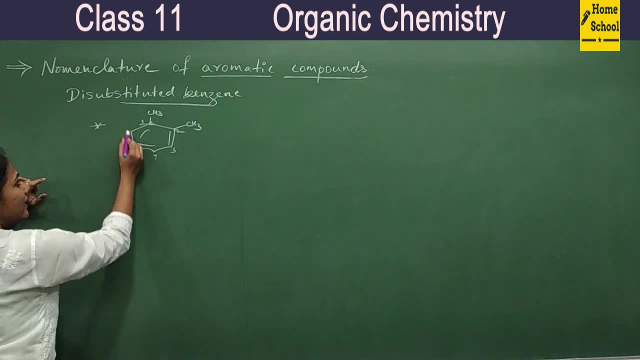 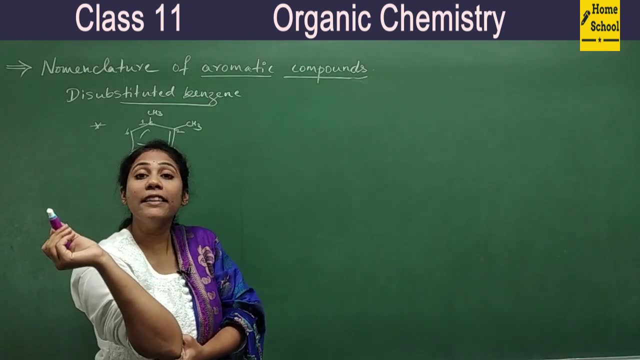 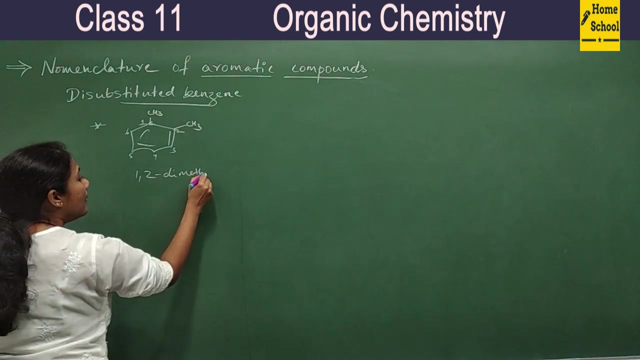 number 2, 3, this is 4, this is 5 and this is 6.. And now both are substituent group. Okay, I mean, you have to mention their name in the form of prefix. So what I can write here: 1, 2 dimethyl benzene. 1, 2 dimethyl benzene. Okay, So this is. 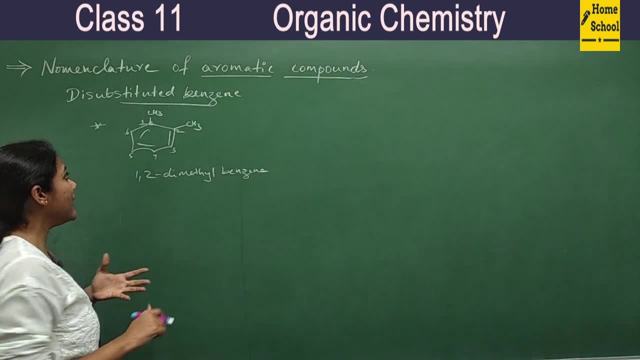 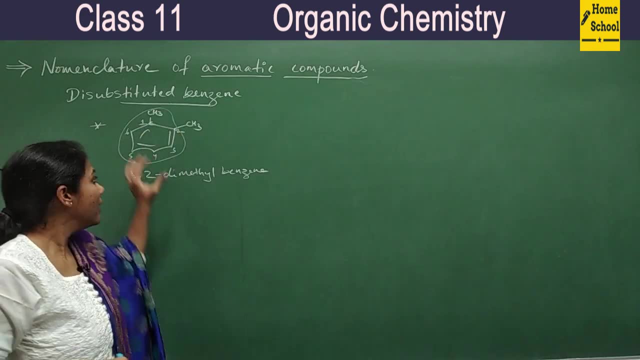 the name, And there is one more way of naming this And if you consider this, this is nothing but toluene, which I told you in the previous case, right? So toluene can be an accepted IUPAC name. 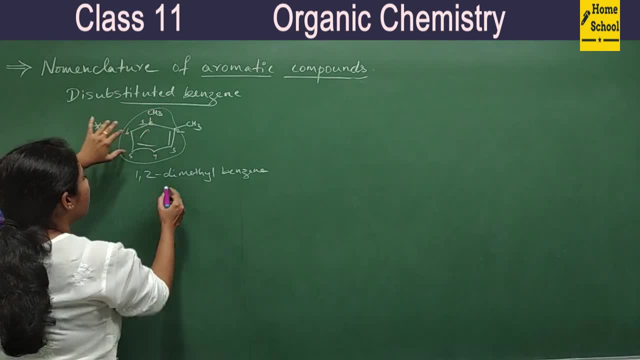 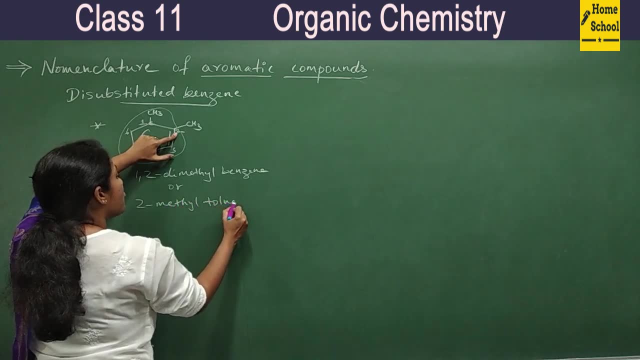 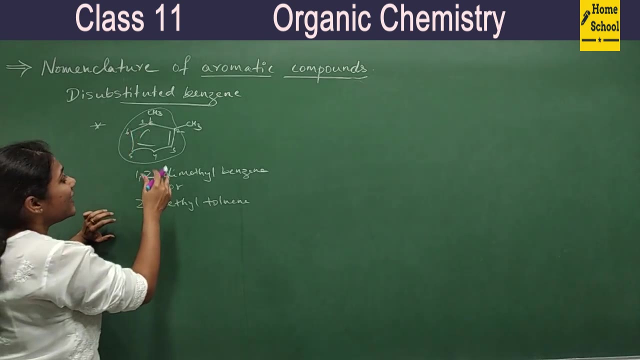 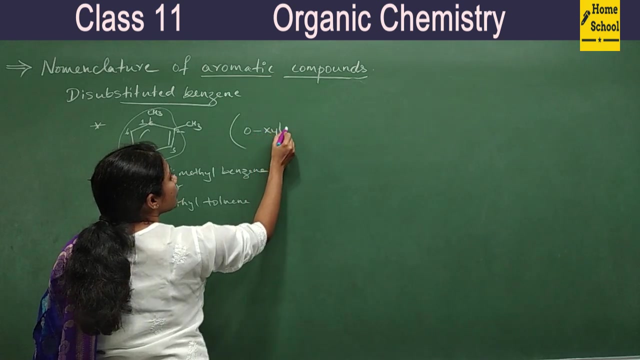 right, So how I can mention its name. I can write it as 2-methyl-2-methyl-toluene, So this is another way of naming this compound, Clear, And these things can be called, as you know, with a common name, orthoxylene. This is: 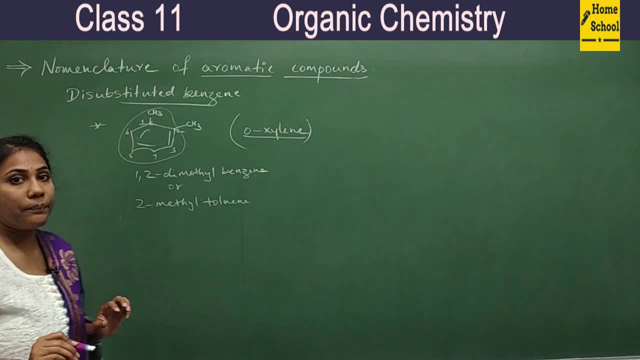 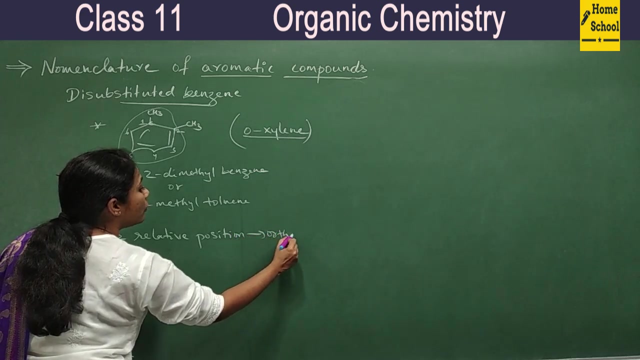 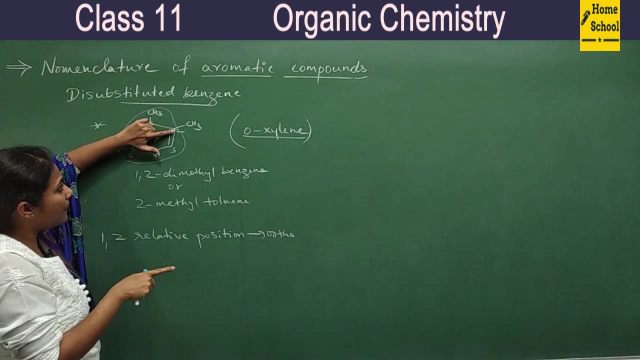 also called with the common name orthoxylene. So O means ortho here. So remember one two relative position. One two relative position is called as ortho. Okay, So with respect to this, another group is in second position. Or if you consider this as carbon, 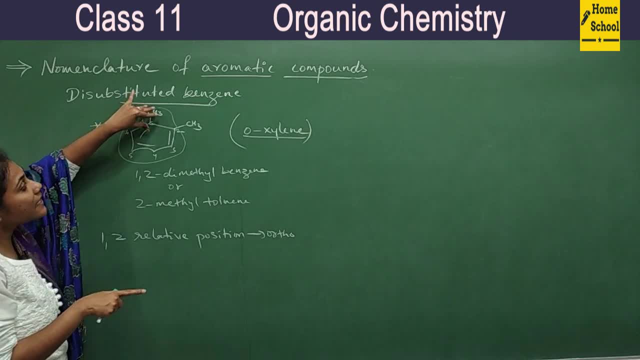 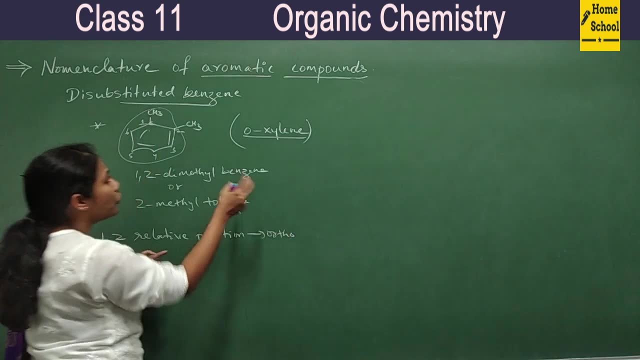 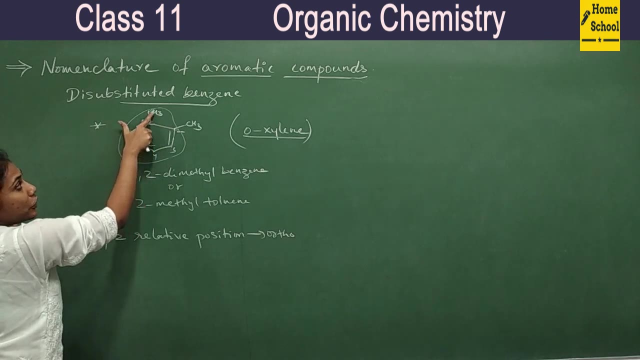 one with respect to this. this group is there in second position, So one, two relative position can be called as ortho position. So they are in ortho. I can say: this is in ortho position with respect to this methyl group. Okay, So that is why it is called. 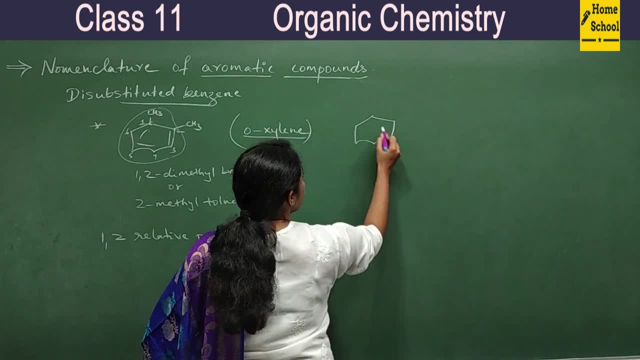 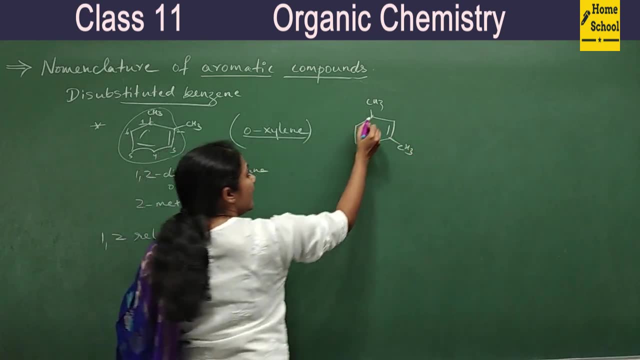 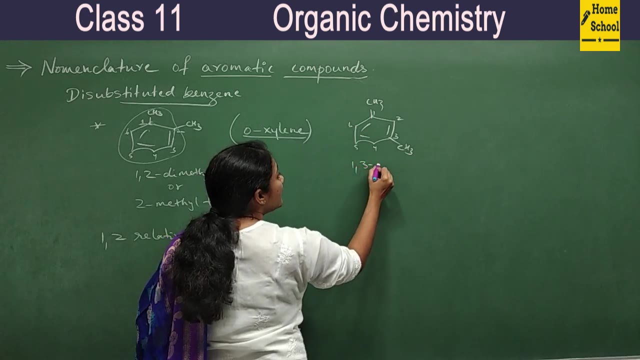 So observe this, Observe this example: CH3, C, CH3 in this position. So what is its name? 1, 2, 3,, 4,, 5, 6.. So this is actually 1,3-dimethyl. methyl benzene, Right, Or I can also call it as 3-methyl toluene, And it has got a common name: metaxylene. Metaxylene, Small m in the sense, meta. Okay, So one 3 relative position is called. 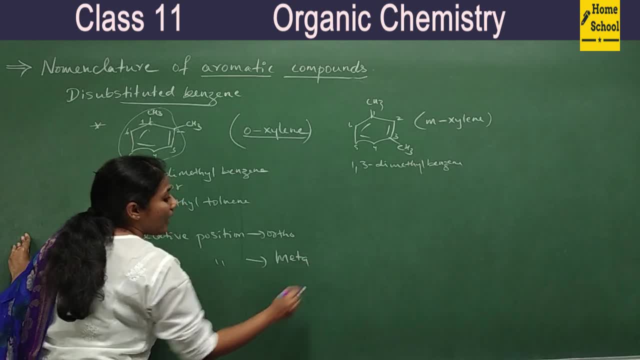 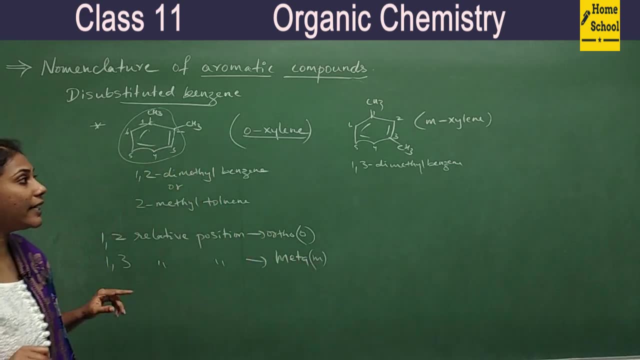 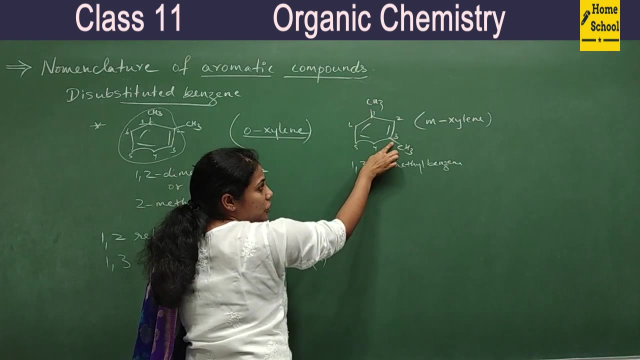 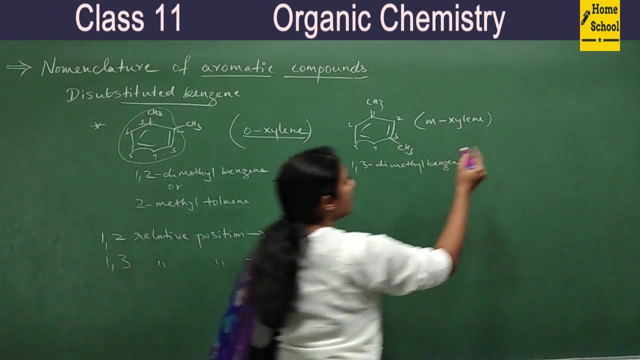 with the term meta. Okay, So ortho is indicated as small o, Meta is indicated as small m. Okay, So if the groups with respect to this CH3, this guy is there in third position- So one 3 relative position is called meta position. Okay, And you observe another example here. You see CH3 and 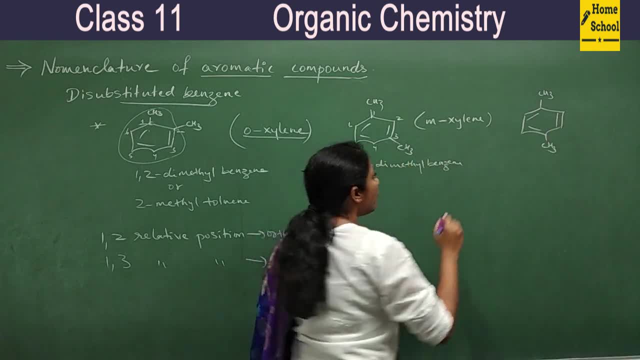 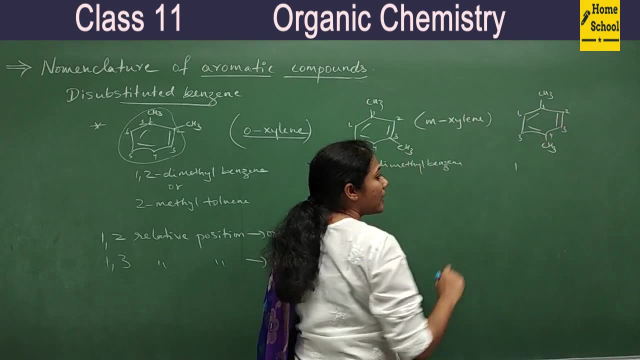 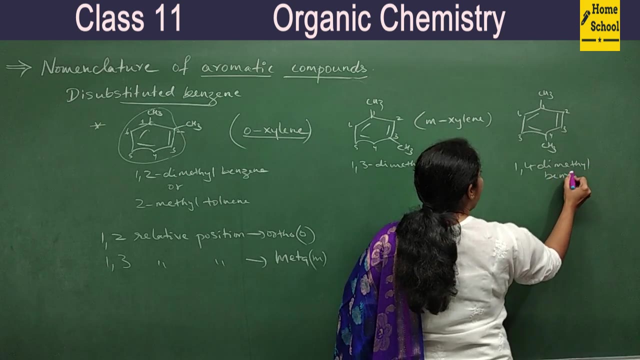 another CH3. I will write here, Okay. So what is the IUPAC name here? 1, 2, 3, 4, 5, 6.. This is a way of numbering. So 1, 4 dimethyl benzene And this has got a common name: paraxylene. This is: 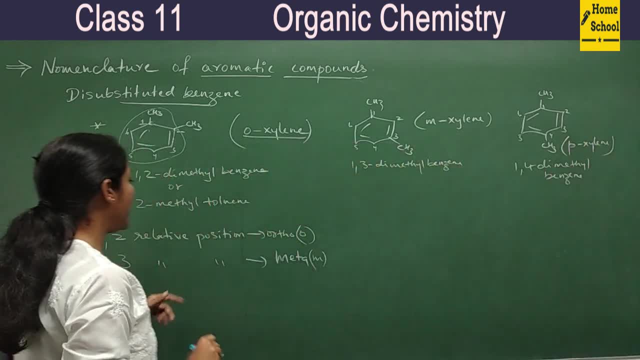 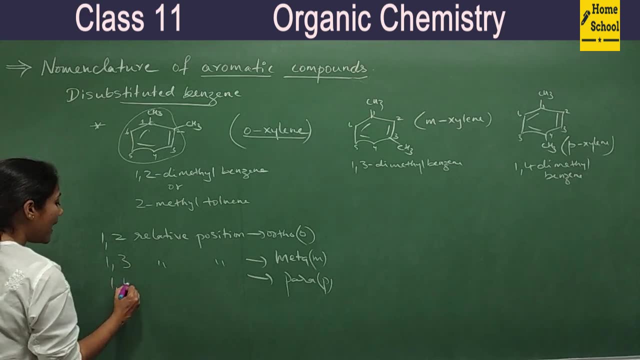 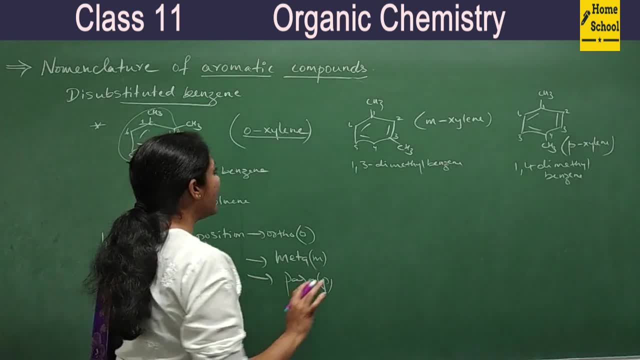 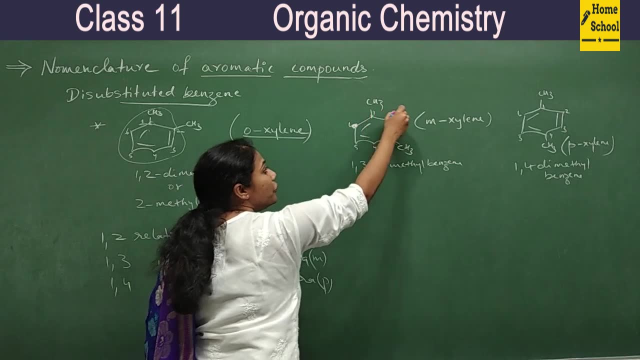 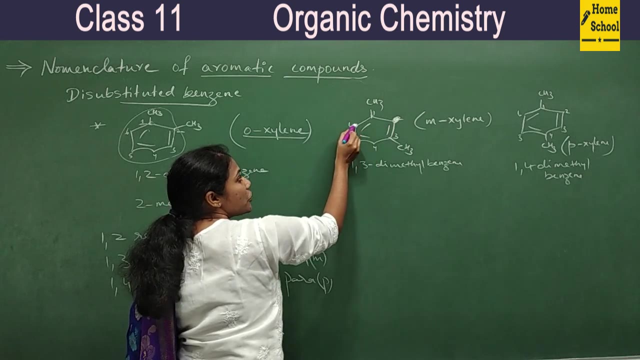 position is para Clear, So always try to remember. you know this position and this position. So, with respect to this, if you number this way, this becomes 2.. If you number this way, by any chance, this position is second position. So these two positions are: 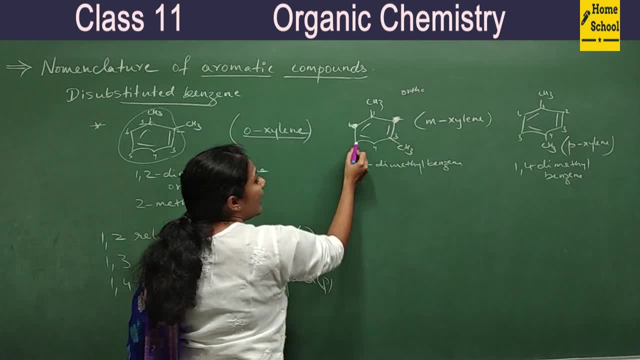 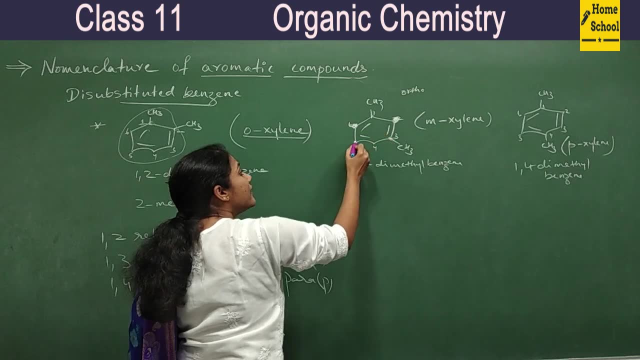 actually ortho positions. Okay, And 1,, 3 position. If you number this way, this becomes 3.. If you number this way, by any chance this becomes 3.. So 1,, 3 relative position is always. 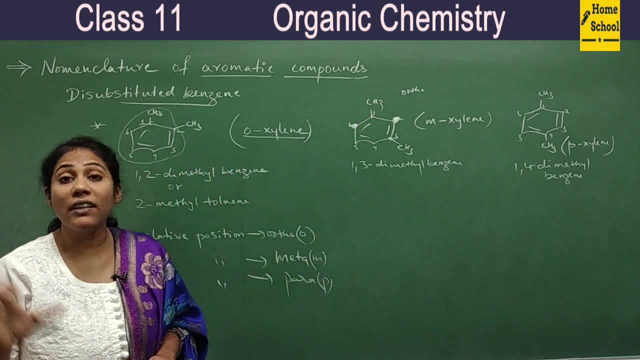 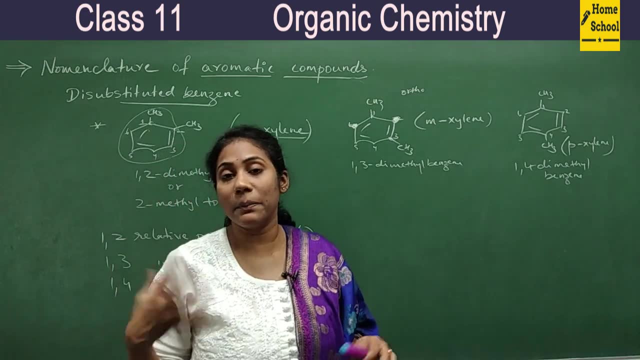 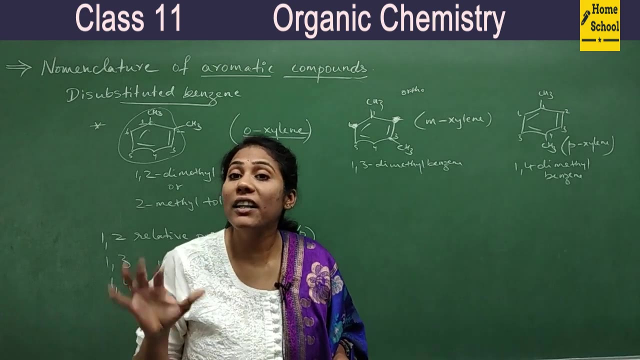 meta And 1, 4. relative position is always para. Okay, So ortho, meta and para is trivial system of naming. That means they are included as common name. Okay, You cannot use ortho, meta and para for IUPAC names. For IUPAC names you have to mention like 1, 4, you know number. 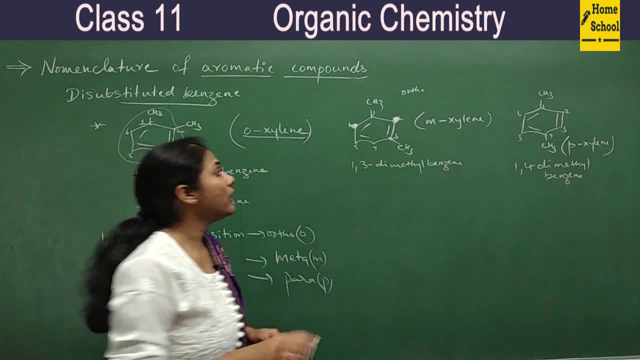 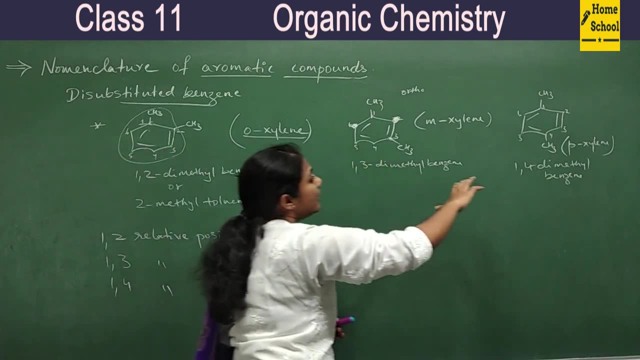 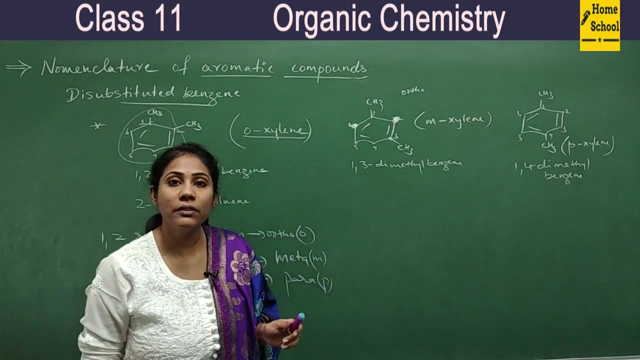 you should mention and then give a name. Okay, So you are not supposed to call it as ortho, meta and para. Okay, So orthoxylene, metoxylene and paraxylene is common names, So it is very important to remember common names also. Clear, Fine, And now let us go for few more examples. 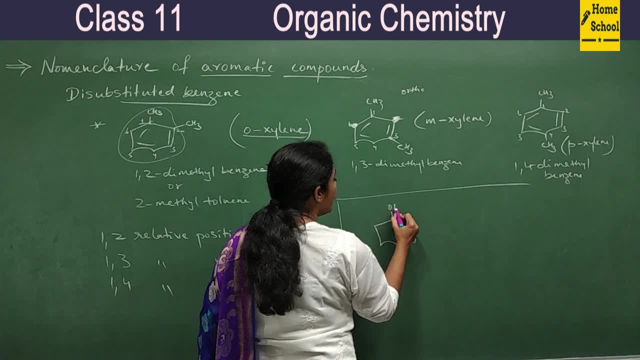 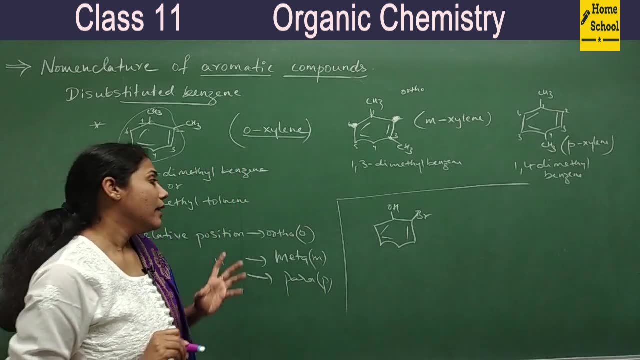 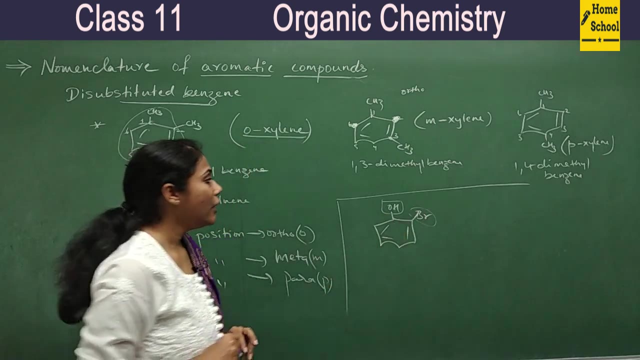 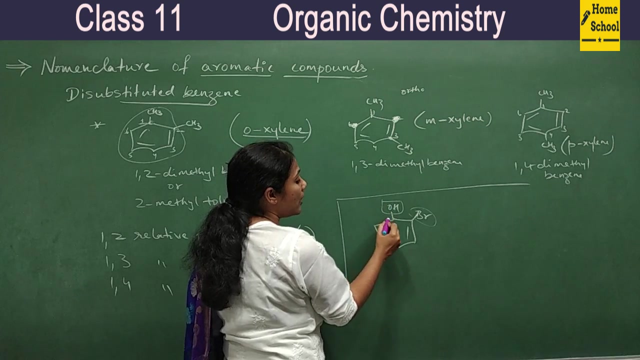 You see this OHBR. So what is the IUPAC name here? Definitely this is a functional group and this is a substituent group, Isn't it? So functional group should be given more preference. So carbon, having a functional group, will get number 1 position. So this will get number. 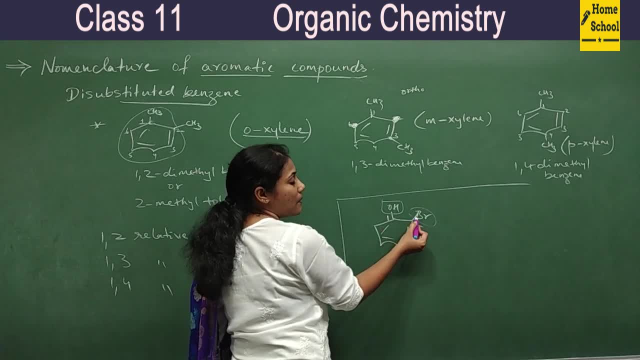 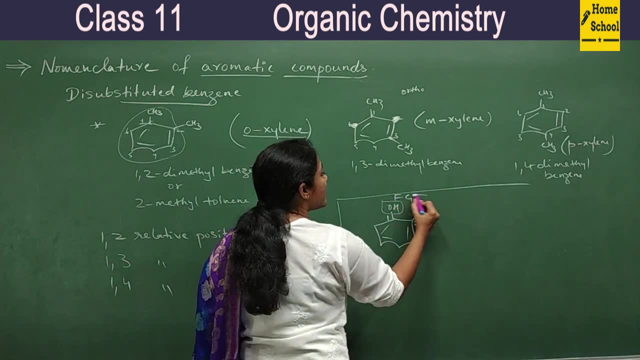 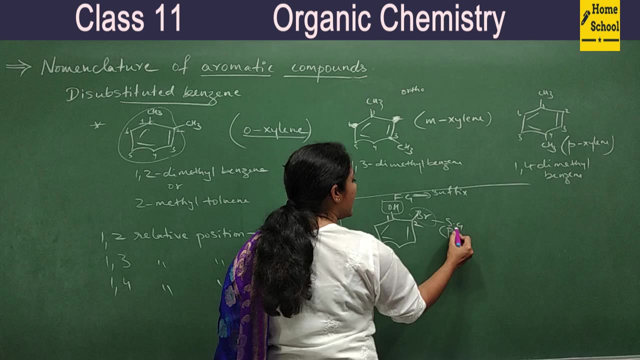 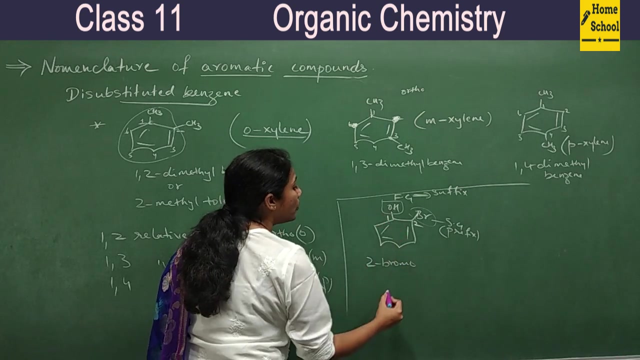 2 position And its name we will write as prefix and its name we will include in suffix, Right? So this is our functional group and its name is written as suffix. And this is our substituent group. Its name is written in prefix. So what is the name here? 2-bromo, 2-bromo benzene. 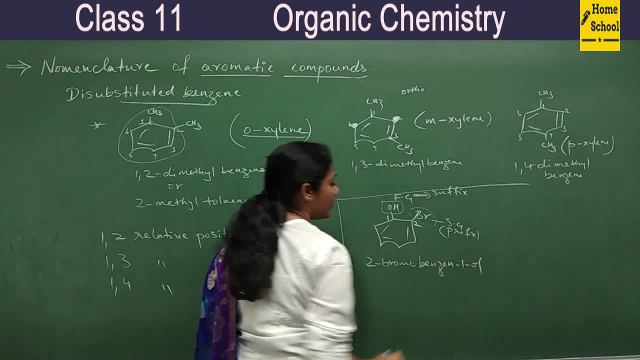 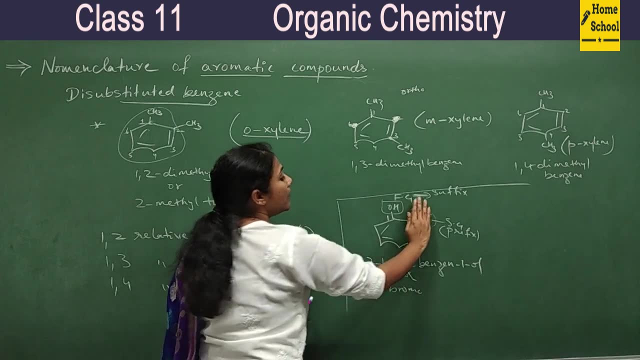 1-ol. Okay, Or we can also write as 2-bromo, 2-bromo benzene, 1-ol. Okay, Or we can also write this as 2-bromo. And if you remove this, I mean if you close this, this is what. 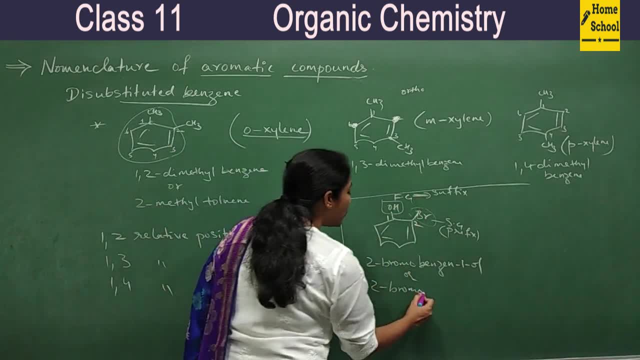 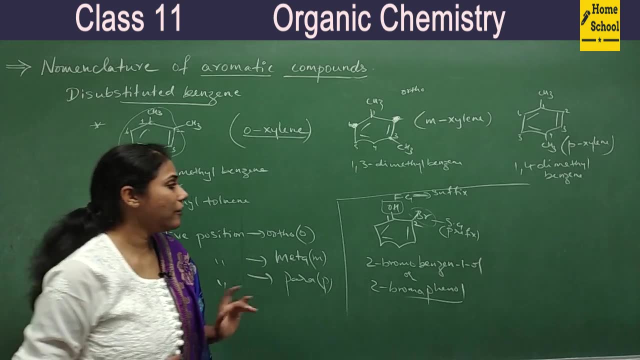 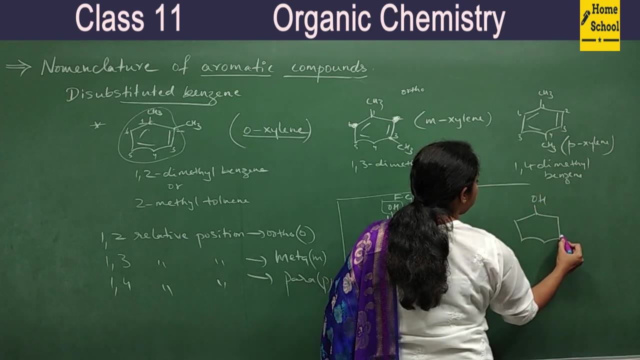 Phenol. Right, We discussed Phenol, So 2-bromo phenol. You can call this compound as 2-bromo phenol also. Okay, Fine, Now let us go for one more example: OHCOOH. So this is the compound. 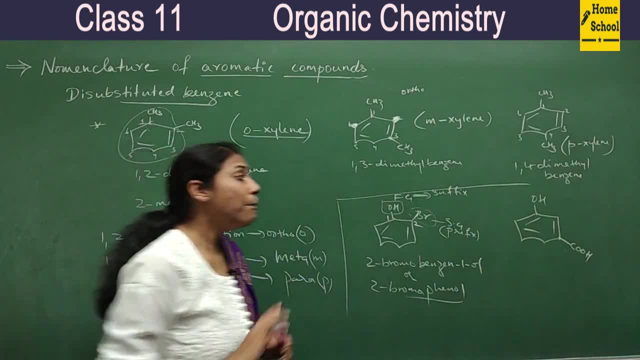 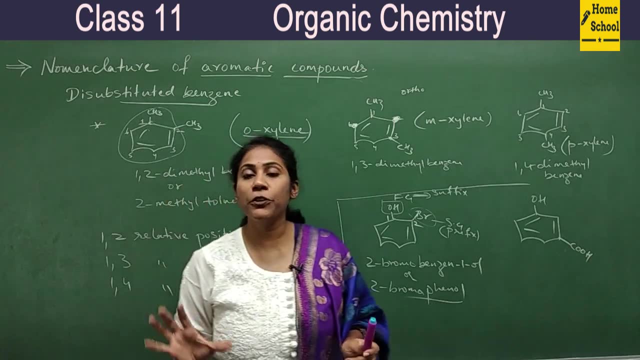 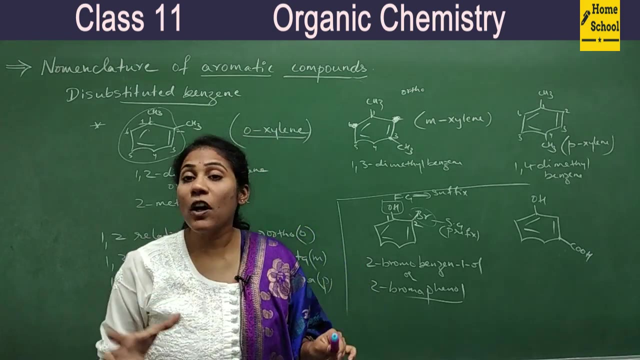 So this is the compound you have. So how do you name this? Both are functional groups. OH is functional group, COOH is also functional group. So when 2 functional groups are there, you have to give priority to one functional group. So according to priority rule that 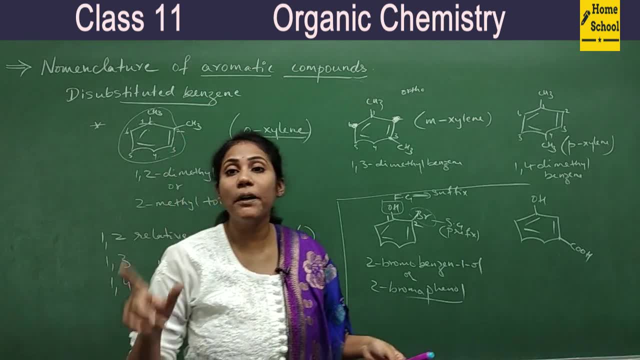 we studied during naming of organic compound having functional groups According to priority rule, who will get more priority? Definitely COOH, Right? So 2-bromo phenol is a functional group, So this is the compound. So how do you name this? Both are functional groups, OHCOOH. 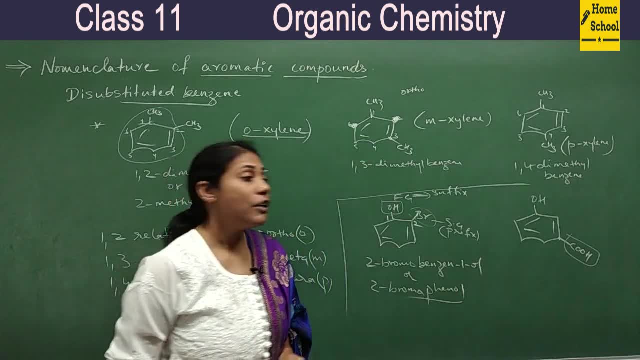 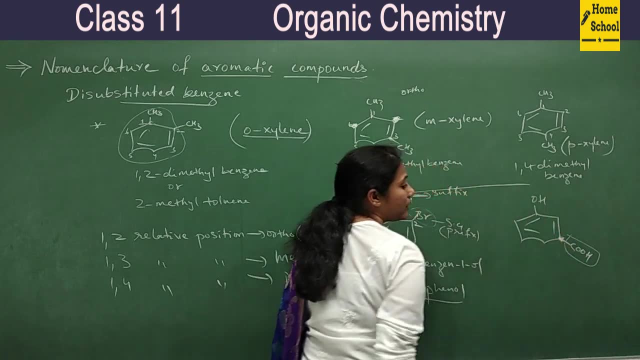 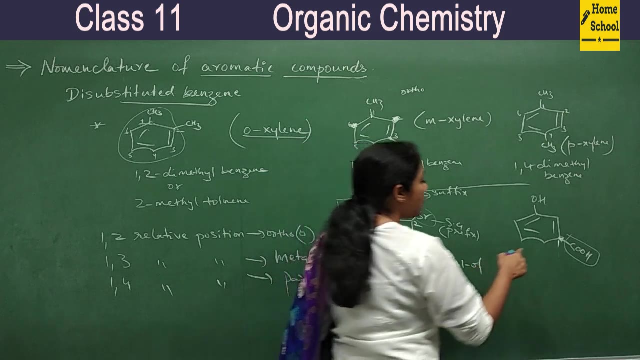 definitely COOH will get more priority. So the functional group which has got more priority is attached to this carbon, So that carbon will get number one position. Okay, So always give number one position for the more prioritized group. Okay, And least priority is this group. 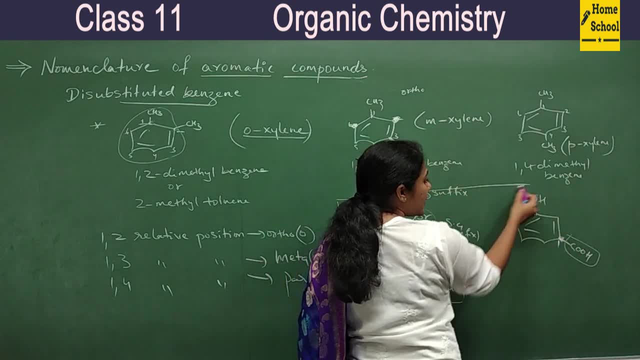 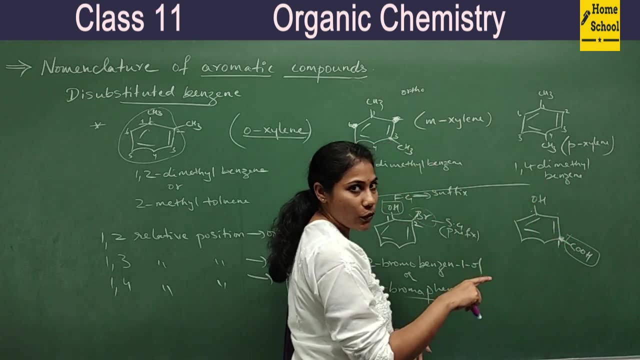 So how do you number it? You can't go this way. If you go this way, one, two, three, four, five you will get. If you number this way, one, two, three. lowest to low count, you have to. 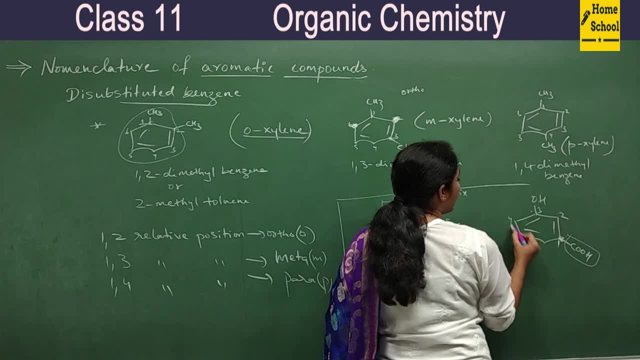 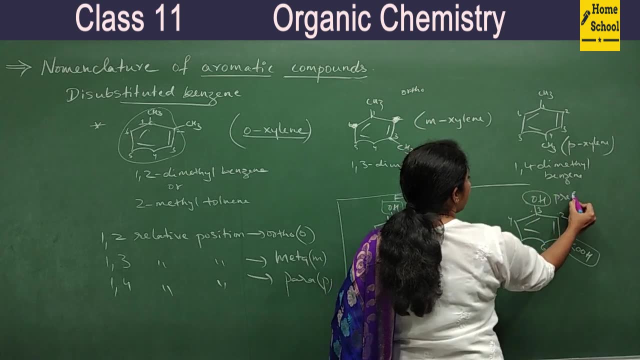 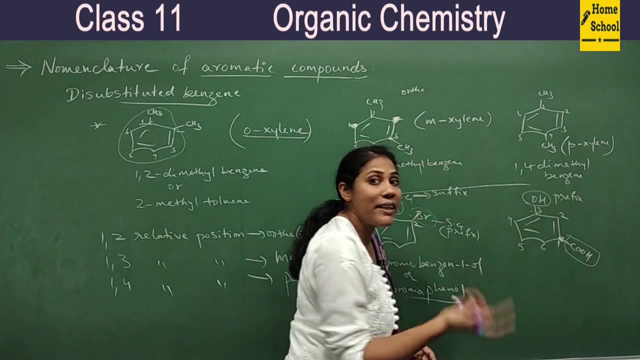 follow. So three is minimum right. One, two, three, four, five, six. This is the way of numbering. Okay, And now this group is written as prefix. So the group which you have given less priority will be written as prefix And the group to which you have given more priority. 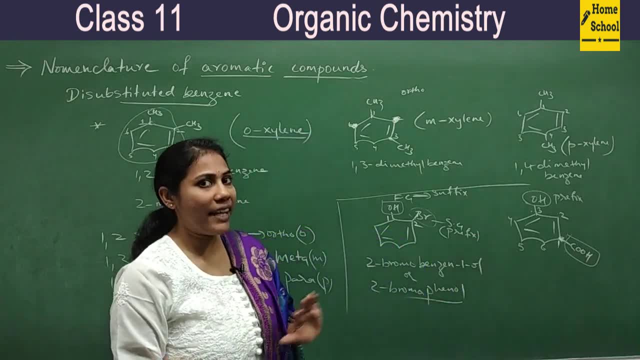 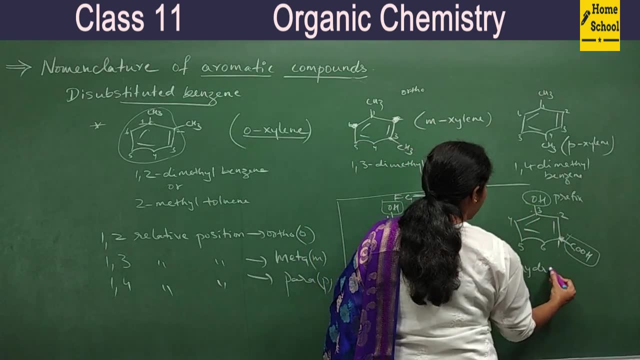 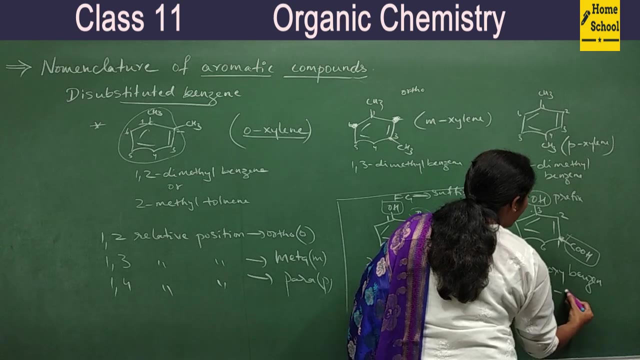 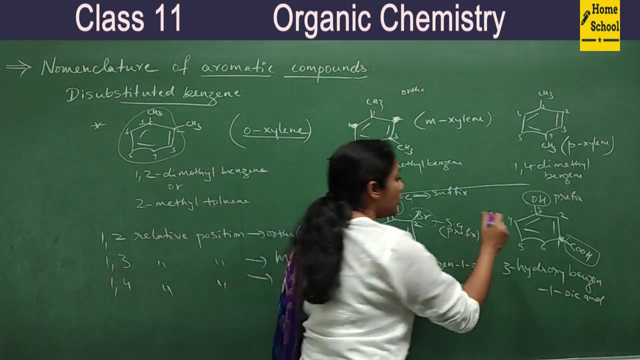 will be written as prefix, So the group to which you have given less priority will be written as suffix. These rules we have already studied, right, Okay? So now what is its name? It is actually 3-hydroxy, 3-hydroxybenzene-1-oic acid, 3-hydroxybenzene-1-oic acid, Or you can also write: 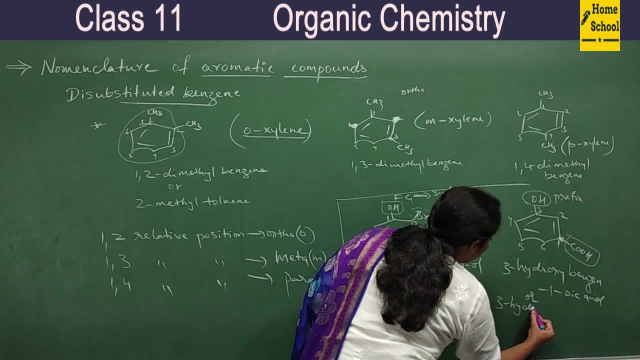 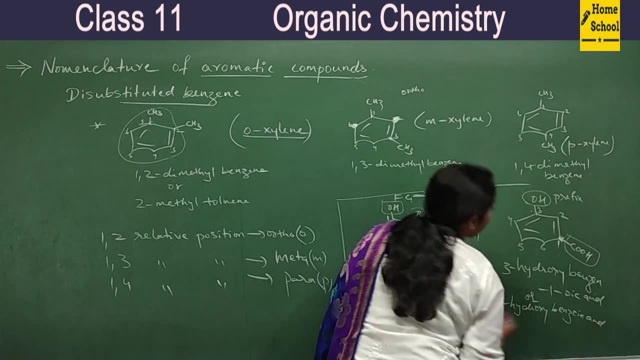 this as 3-hydroxy 3-hydroxybenzene-1-oic acid, Or you can also write this as 3-hydroxy 3-hydroxybenzoic acid. And if you close this, what is this? This is like benzoic acid, So. 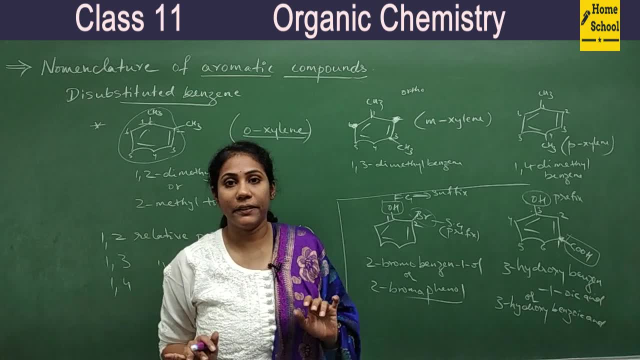 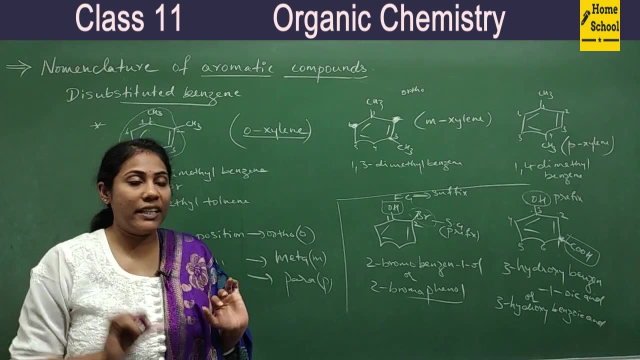 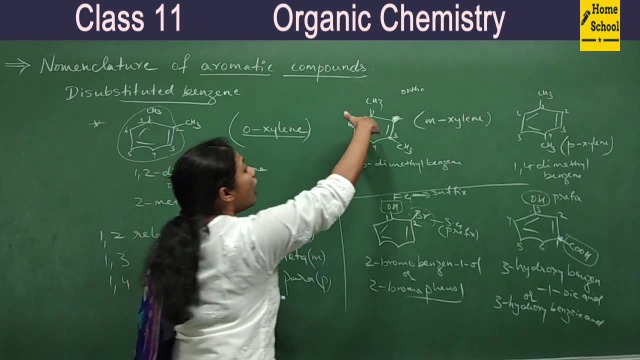 3-hydroxybenzoic acid. That can also be correct. Okay, So this is how you will name disubstituted benzene. Okay, Fine, And now we will see the nomenclature of benzene, which is having a long 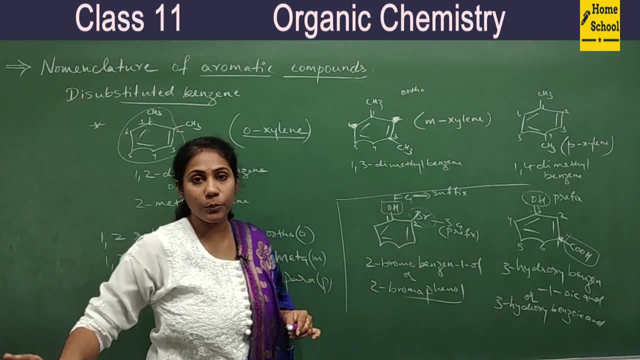 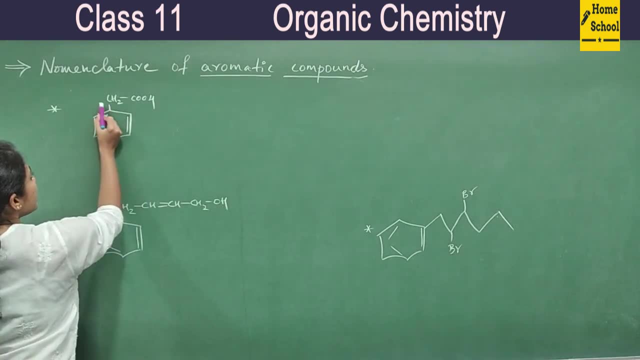 side chain, alkane side chain with functional group. That is also very, very important. See these examples that I have written on a board, guys. You see side chain. Okay, Some alkane side chain as a functional group and bigger side chains- All these are very, very big side chains. 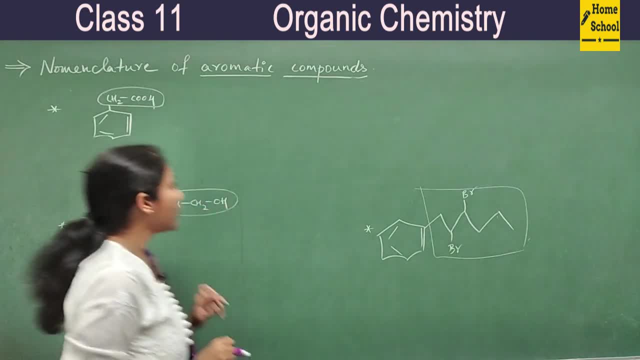 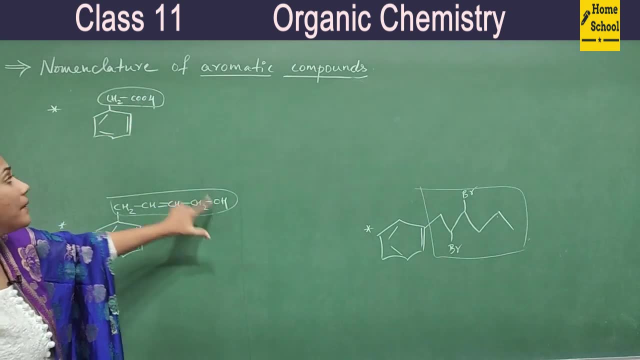 Right. So when you have this long side chain, if the side chain has a double bond, or if the side chain has functional groups, something like that, then you have a long side chain, So you can like this. Then benzene ring must be considered as substituent group. Okay, So you are not supposed. 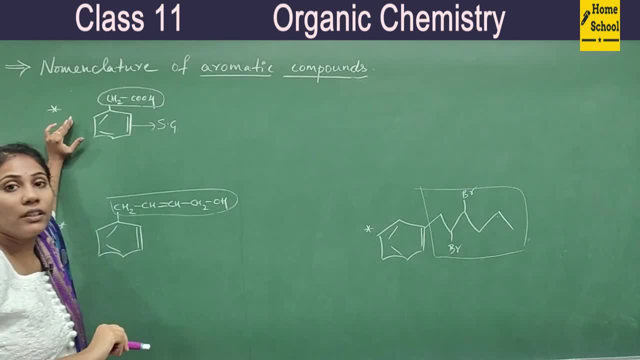 to write benzene as word root, You have to take the benzene ring and write its name in the form of prefix. Okay, So this becomes your main chain. To this main chain, benzene is just like a branch, It is just like a substituent group. Okay, So this is. 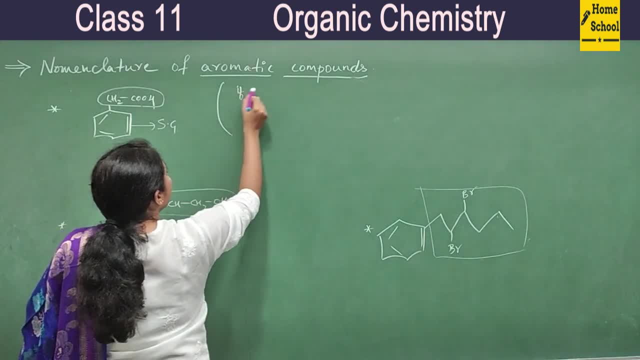 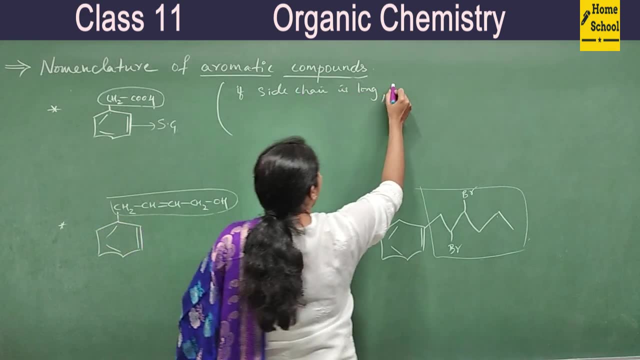 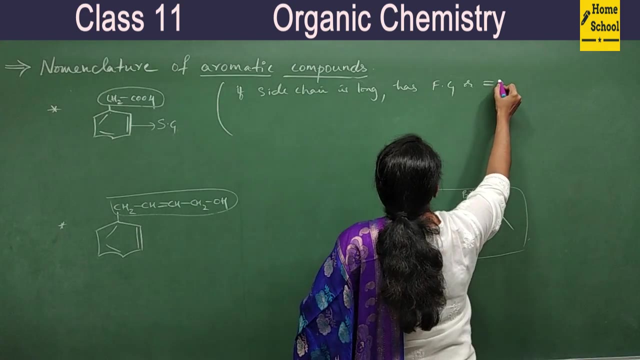 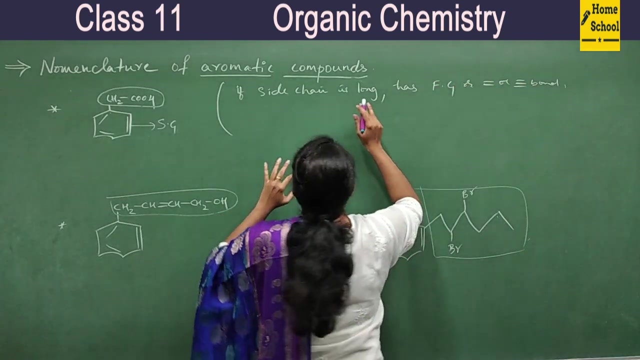 one of the very, very important rule. So what is the rule If side chain is long or if it has functional group or double or triple bonds? What Side chain If has double bond, triple bond or functional group, Okay, Then it is parent chain. 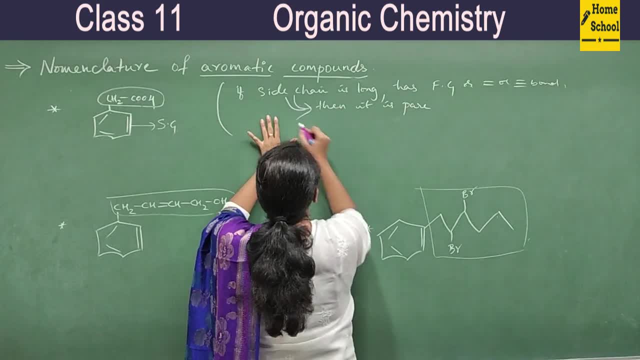 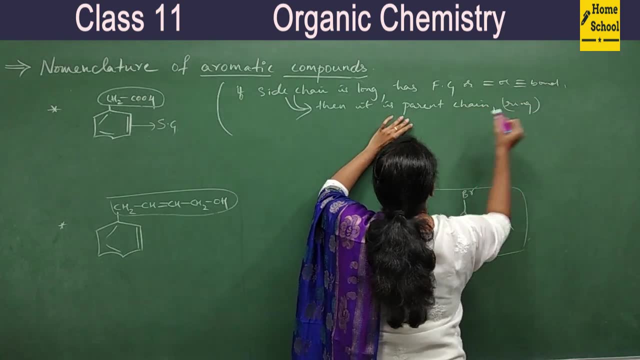 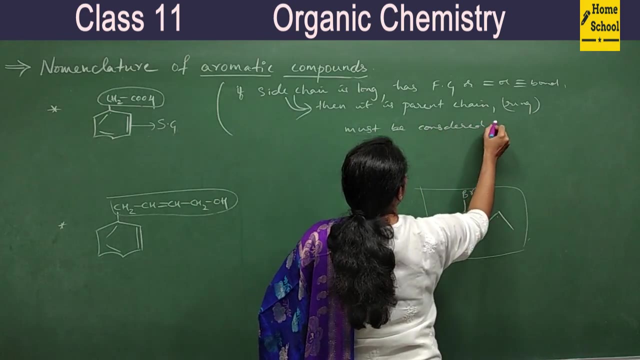 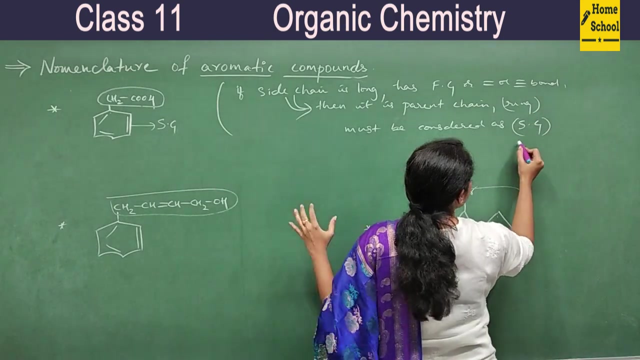 It is in the sense side chain is parent chain. Ring, that is, benzene ring, must be considered. must be considered as substituent group. Okay, And its name, the benzene name, should come in the form of prefix Right. Hope you can understand the point. 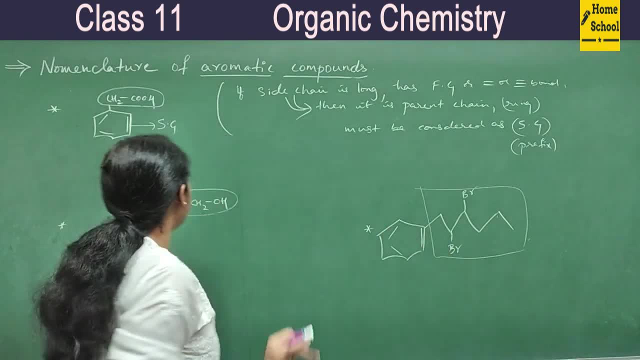 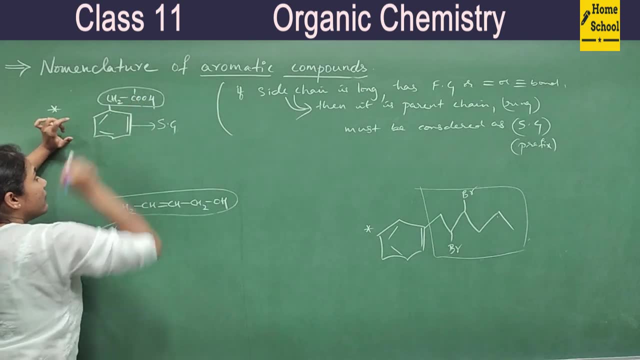 This is what I am telling you. This is really very important. See how I name this. So this is my parent chain Functional group containing carbon should have number one, position Right And the next, carbon. this is number two. So this is like a branch. This is like a branch And you are mentioning 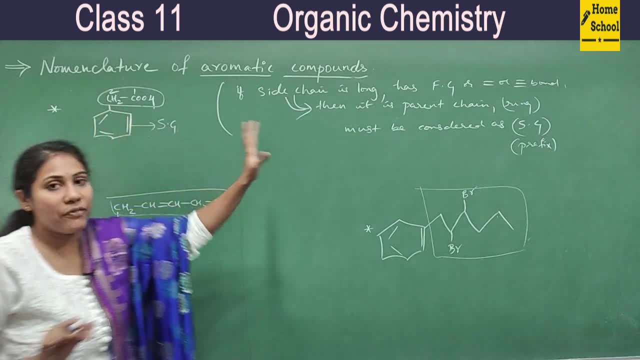 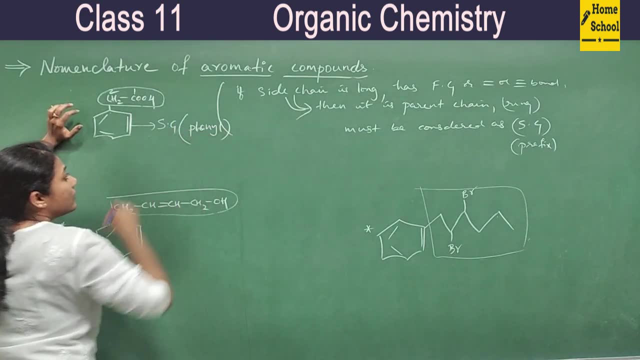 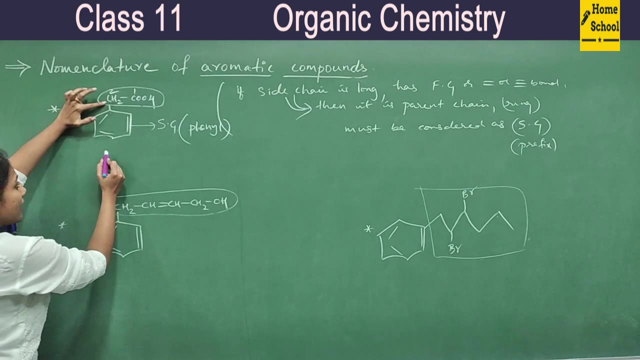 this branch name this benzene name in the form of prefix. So when you write benzene as a prefix, you have to use the word phenyl, don't use the word benzyl, we have to use the word phenyl. So how do I name this? It is actually. 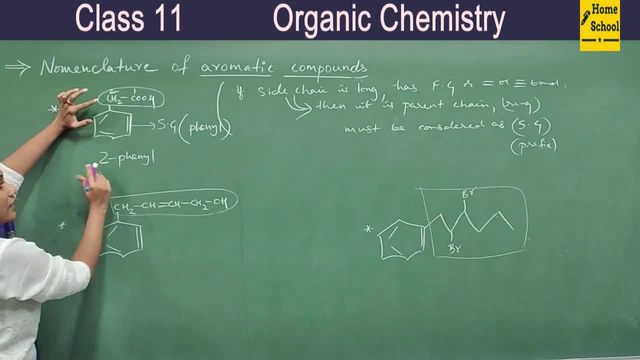 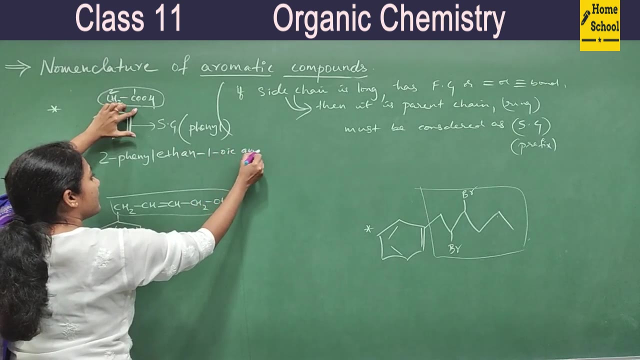 2-phenyl, 2-phenyl. this much is the prefix, Now word root. See the main chain has two carbons, So word root is eth, and between carbon single bond, So N hyphen 1-oic acid. Okay, So it is. 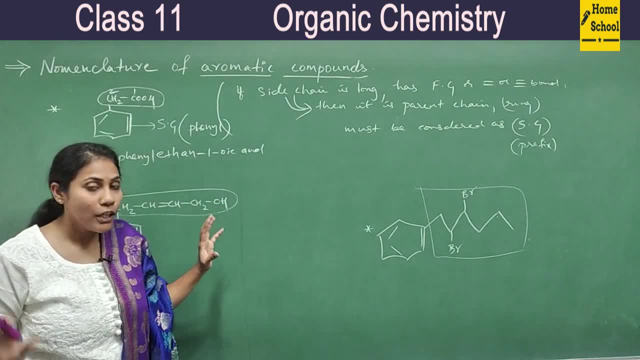 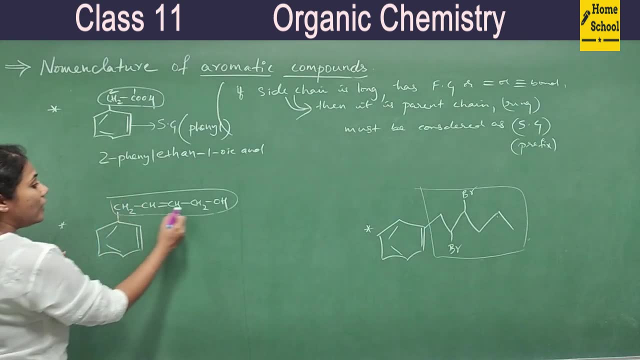 2-phenyl-ethanoic acid. Right, So hope you are clear how you have to name such compound. Coming to this compound, you see it is a long side chain, It has got double bond, it has got functional group. So this is your parent chain and this is going to be the substituent group. 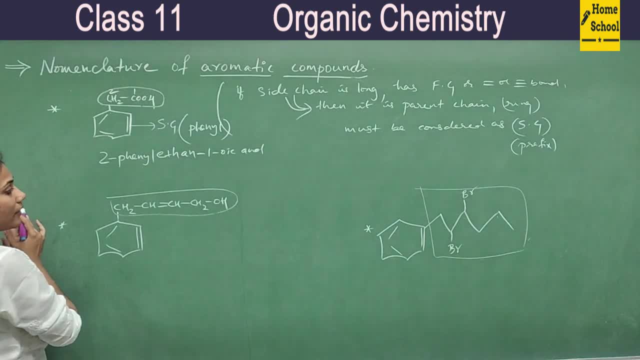 Okay, So how do you number this? How do you number? So? functional group containing carbon should have more preference, So that carbon gets numbered Number 1 position, this is number 2,, this is number 3,, this is number 4.. So here, what is the? 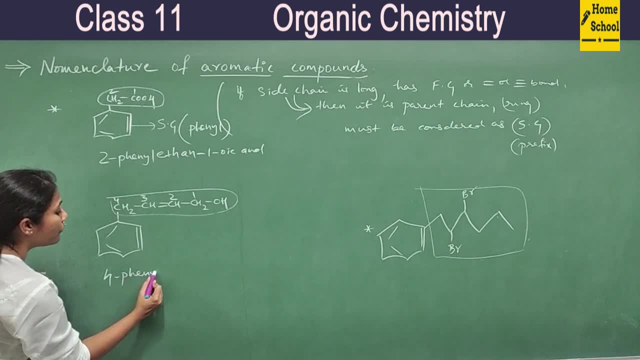 name 4-phenyl, 4-phenyl over branch name. we have finished in prefix, Now word root: Parent chain has got four carbons. So bute, all single, sorry bute- and you have a double bond You don't have. 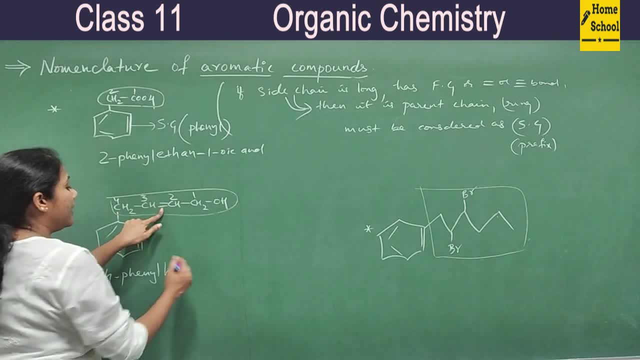 all single bonds, Right. You have a double bond at which carbon Second carbon, So hyphen 2-en-1-ol. Okay, So 4-phenyl bute 2-en-1-ol is the IUPAC name of this compound, Right, Fine? 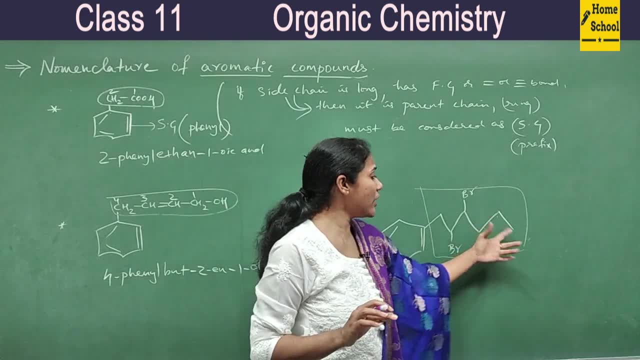 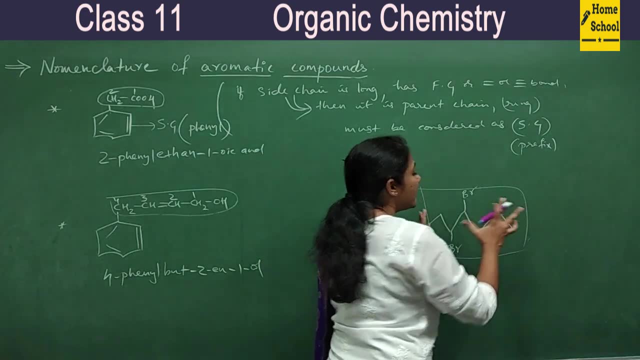 Coming to this compound, you don't have any functional group, But you see, it is a long chain with two branches. So even then, you have to consider this as your parent chain and this is going to be a substituent group. Okay, 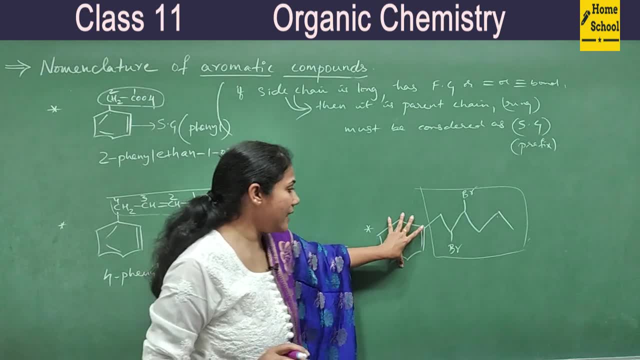 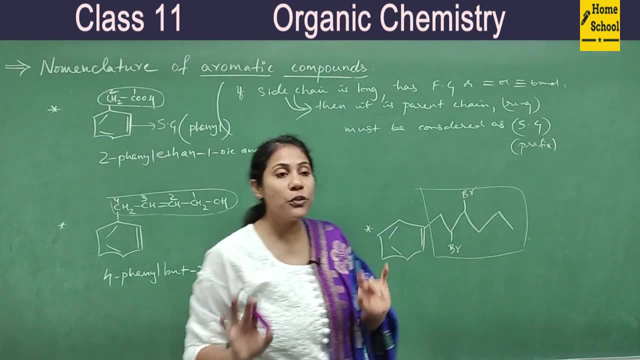 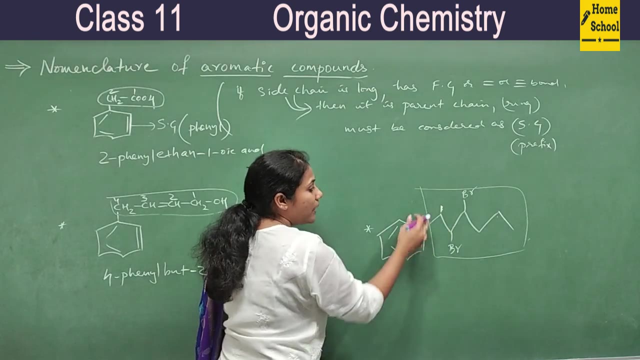 So now you have a substituent group as benzene. Another substituent group is bromine. The third substituent group is also bromine. So from which carbon onwards you will number. So this is your first carbon. Okay, So you are giving more preference to benzene substituent group. So 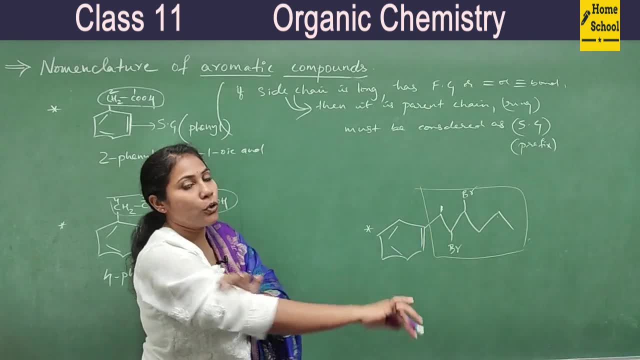 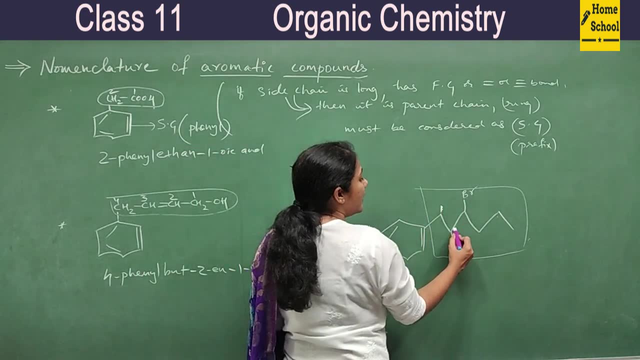 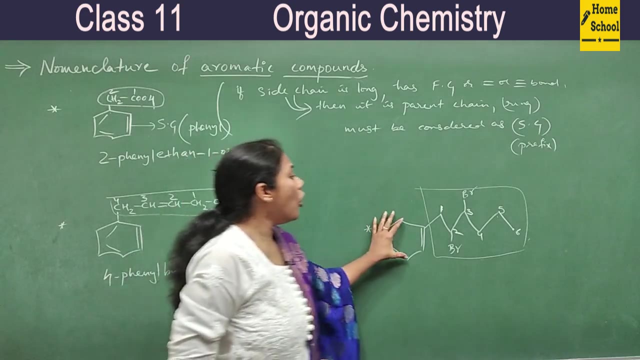 this is your first carbon, or you must actually follow the lowest locant. Lowest locant, if you follow, numbering must go from left to right, in this case, Right. So this is number 1, this is 3, this is 4, this is 5 and this carbon is 6.. Okay, So now all these guys are prefix writing. 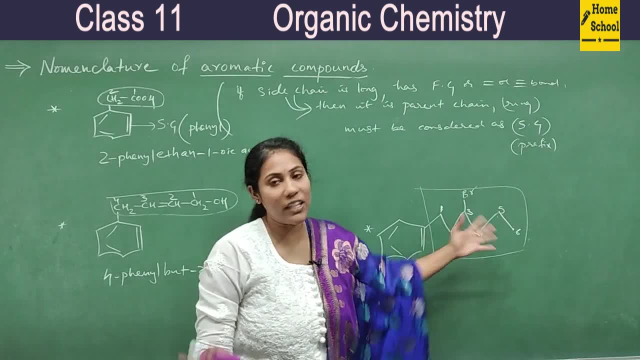 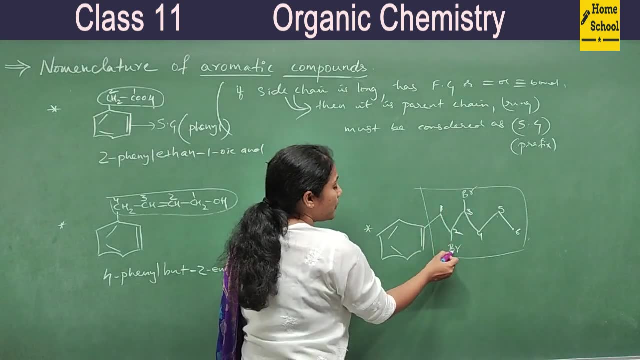 group. I mean you have to mention their name in prefix. There is no functional group to write as a suffix, Right? So bromo, bromo, It's name is bromo and this is phenyl, So alphabetically, 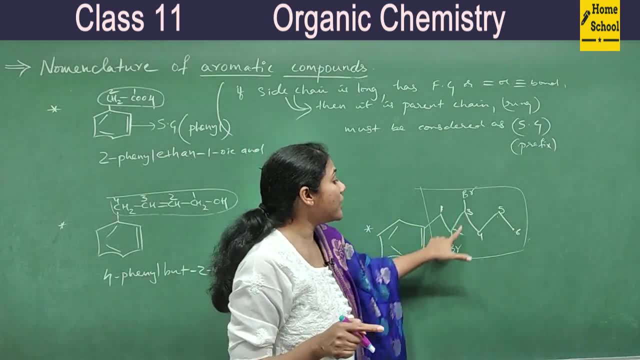 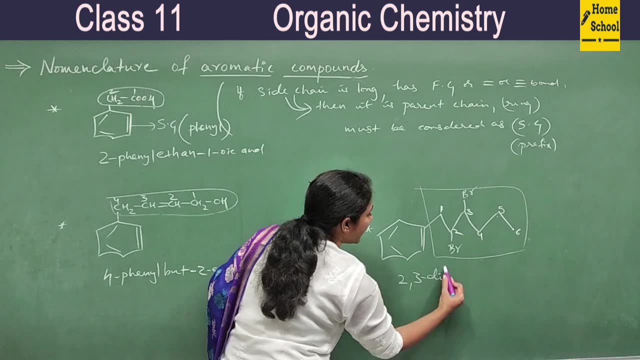 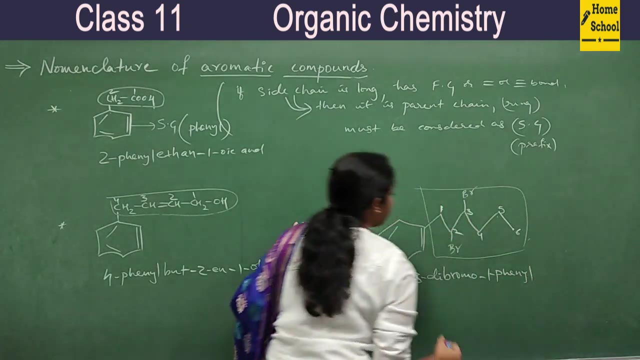 who will come first? Bromine will come first, So you have to mention bromine first. Two bromines are there at second carbon and third carbon. So it is 2,3-dibromo, right. 1-phenyl, 1-phenyl. and then how many carbons in a chyne, 6 carbons. 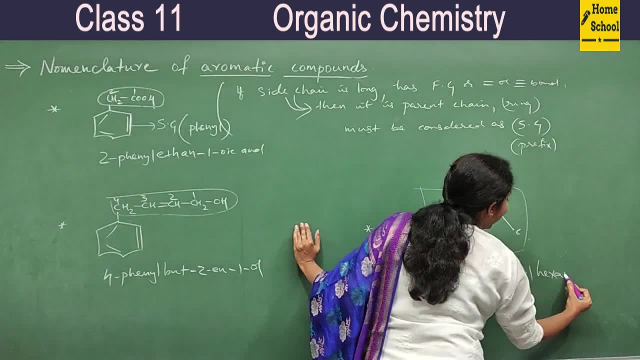 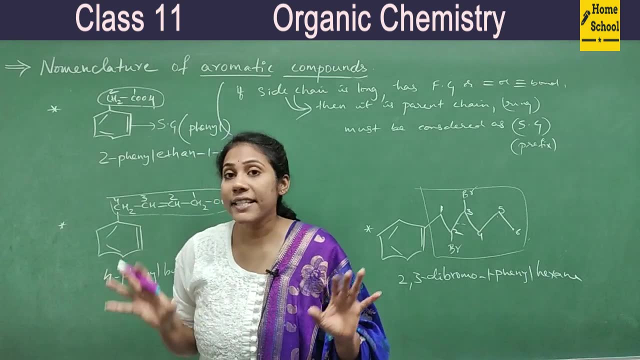 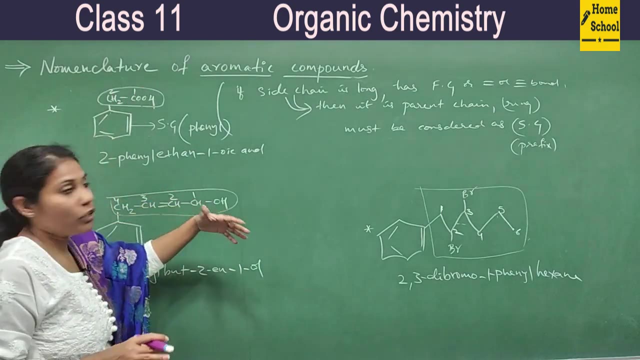 So hex and all single bonds, hexane, 2,3-dibromo 1-phenyl hexane is the name. Okay, So this is how you have to name aromatic compounds which had got a side chyne, Okay So. 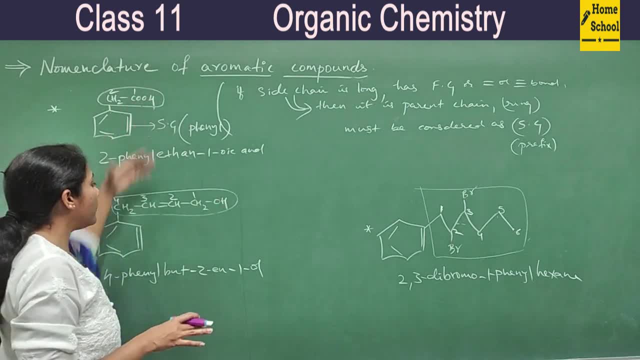 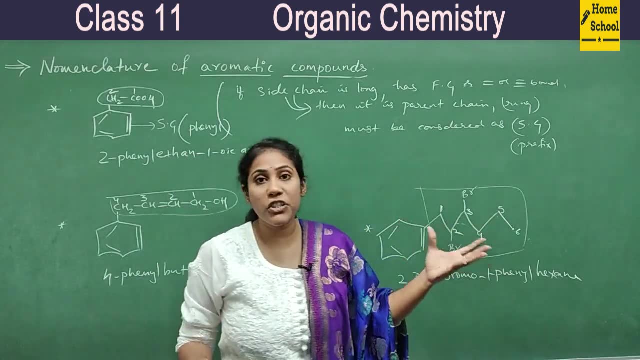 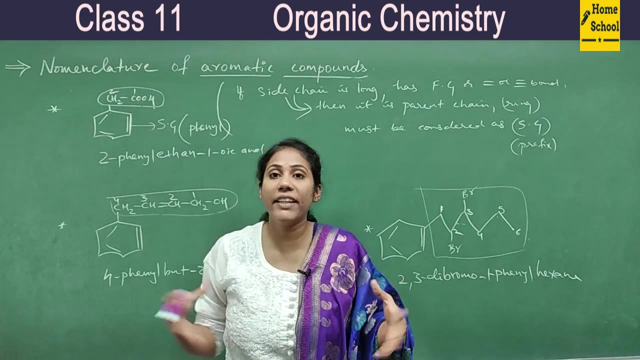 if the side chyne is having a functional group, or if it has unsaturation, or if it is some branched hydrocarbon chyne, then that is your parent chyne. and benzene is considered, as you know, branch or substituent group. So that way you have to name. Is that clear? So 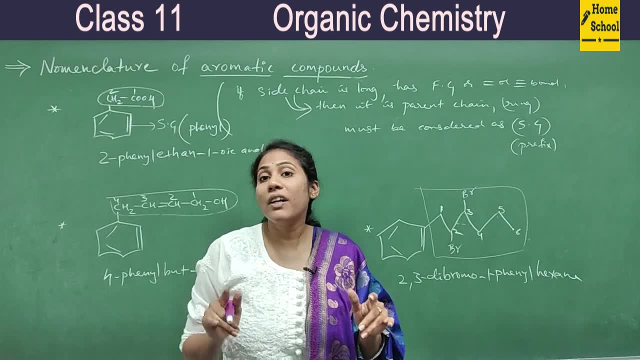 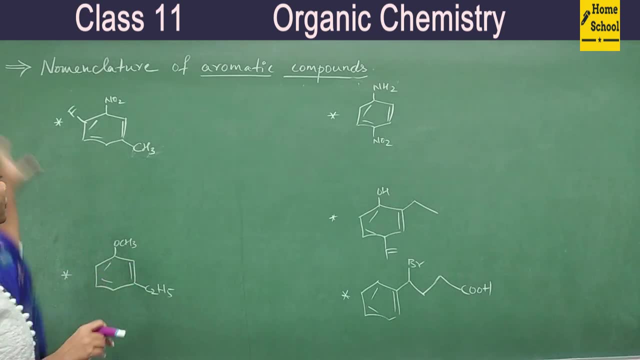 hope you have understood this video. If you have any questions, please do not hesitate to comment below. Hope the concept has become very much clear Now. we will work with few more examples. See guys, these are few more examples. We will try to name them. If you look at the first, 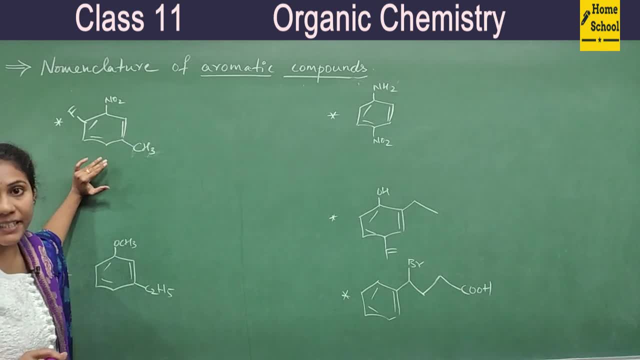 compound. I have three substituent groups on a benzene ring right. So here the big question mark is for which carbon you will give number one position. All the three are substituent groups, So for which one you give more preference? 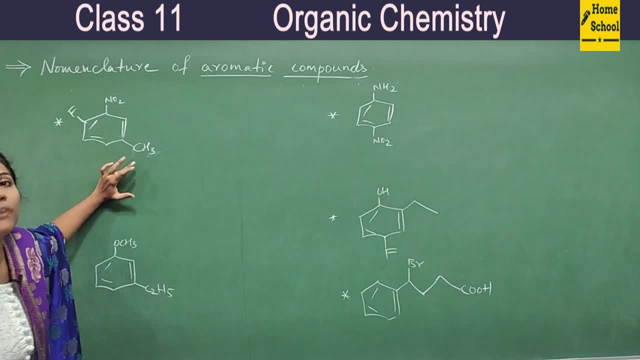 So in that case, go according to alphabetical order. Okay, So its name is fluoro, This is nitro, This is methyl. So fluoro comes first, isn't it? So give number one position for this particular carbon. So now, lowest to low, control you follow. So how do you give number? 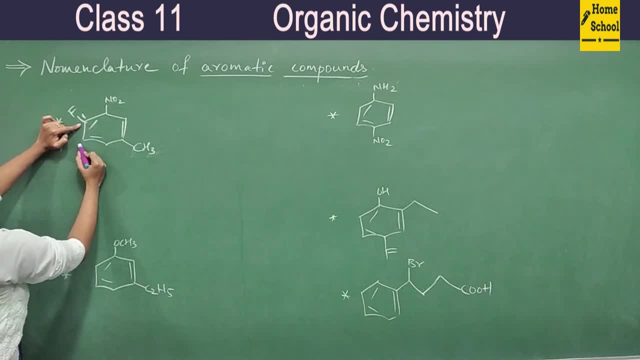 If you can't go from this side, 1,, 2,, 3.. So if you go from this side, 1,, 2,, 3,, 4,, 5, 6.. What is the lowest to low count you will get. You see, 1 plus. what is the low count here? 1 plus 4 plus. 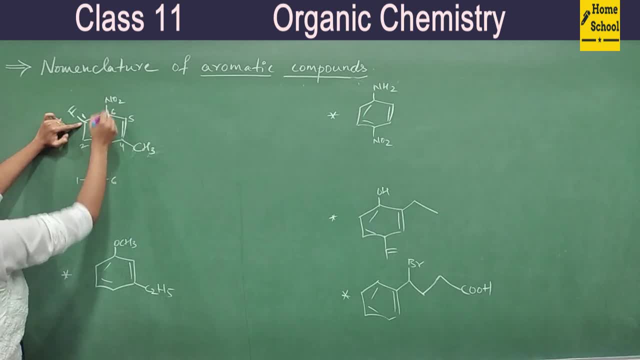 6. At fourth carbon, this group. sixth carbon, this group. right, So it is 11.. If you add these numbers, you will get 11.. But if I follow the other way of numbering, say if I give number, 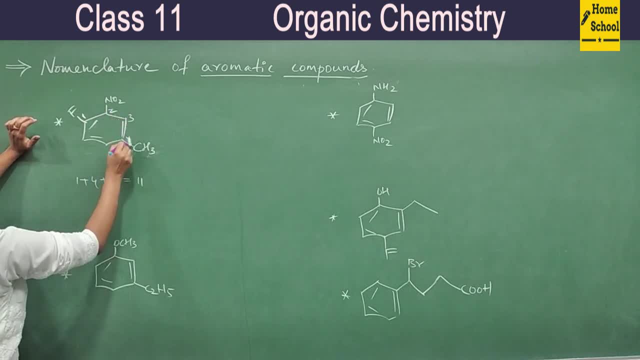 two, position for two for this carbon: 3,, 4,, 5,, 6.. So what is the low count? you will get 1, plus 2 plus 4, right, You will get you know 4 plus 2, 6, 6 plus 1, 7.. So lowest to low count. 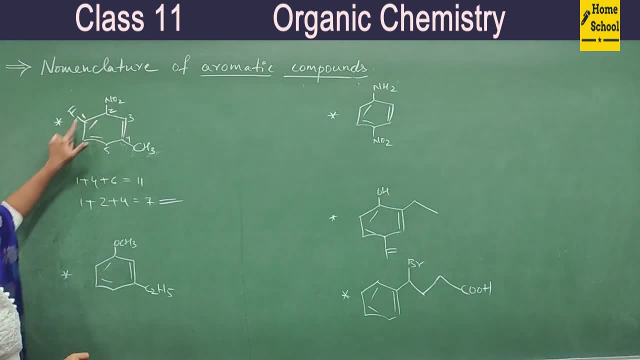 is this way of numbering right, So we will follow this way of numbering. So now numbering is given. Now you just have to write its name. So all the three names you have to mention as a prefix. So how do you mention? Go according to alphabetical order. So it is 1, fluoro. 1 fluoro. then comes methyl, right. So that is 4-methyl-2-nitrobenzene. okay, So 1 fluoro, 4-methyl-2-nitrobenzene is the name of this compound, right? So this is how you have to. 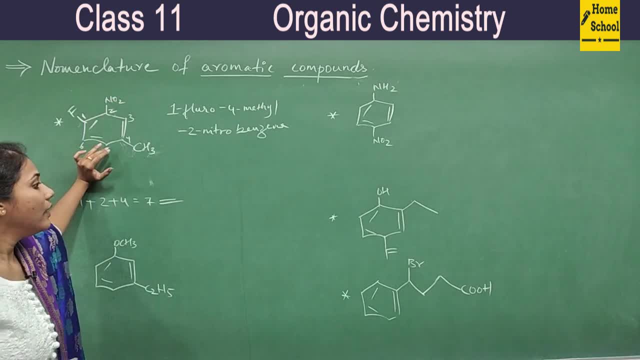 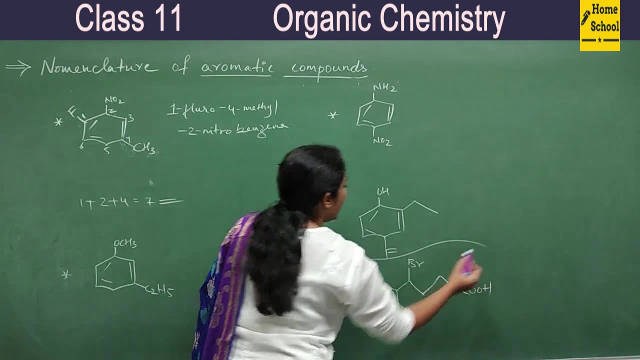 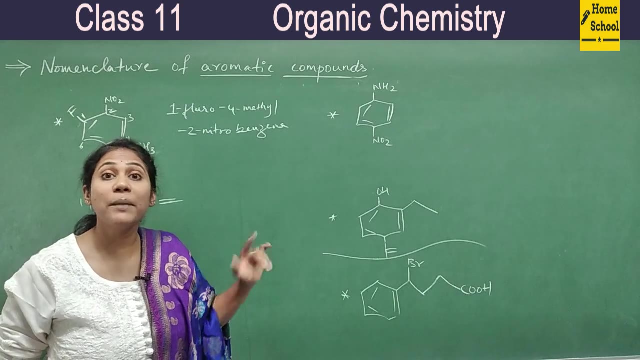 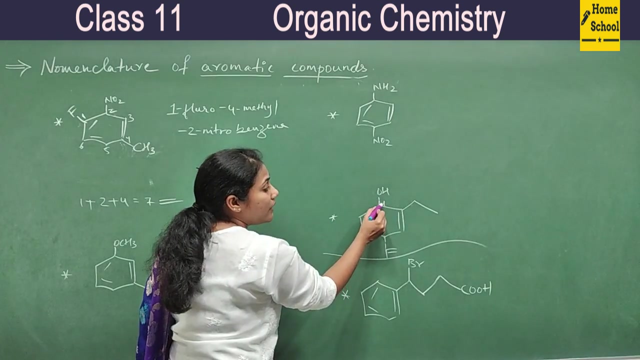 name. if three substituent groups are there And among the three if you have any functional group, look at this compound. Here also three substituent groups are there, But among the three one is a functional group, that is OH. Then more preference is always for the functional group. So here this OH containing carbon will. 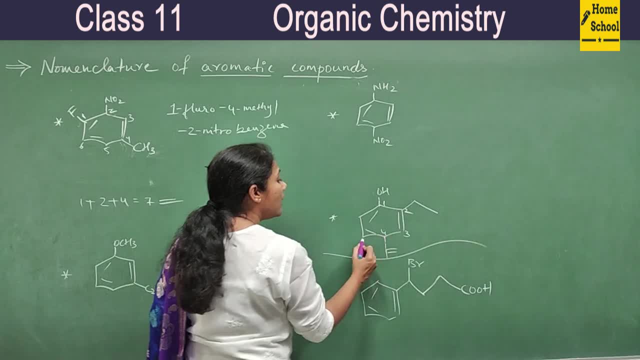 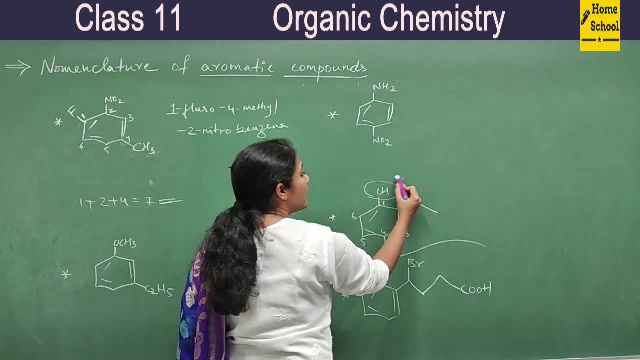 get number 1 position, This is 2,, this is 3,, this is 4,, 5 and 6, okay, So now, what is its name Here? its name you will mention as suffix, because it is a functional group. Now, this is branch. 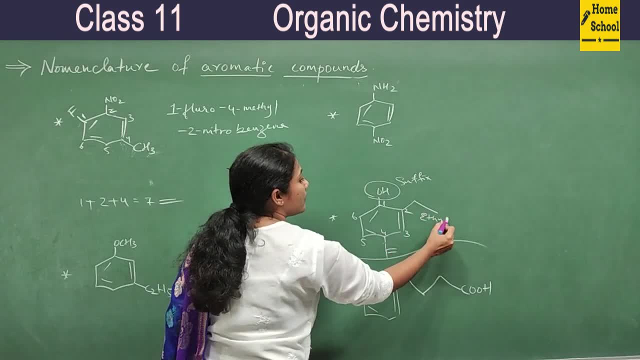 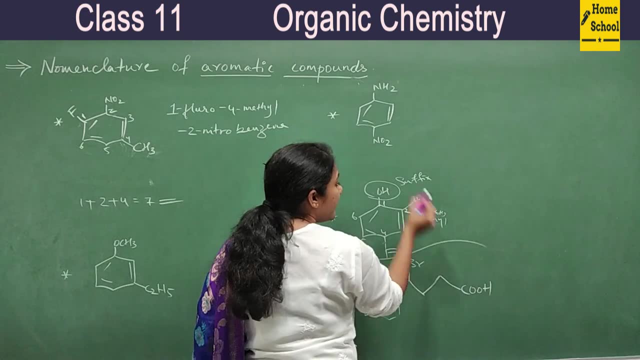 this is branch substituent group, This is ethyl right, CH2,, CH3, ethyl And this is fluoro. So, alphabetically, which comes first E comes first right. So how do you name this 2-ethyl? 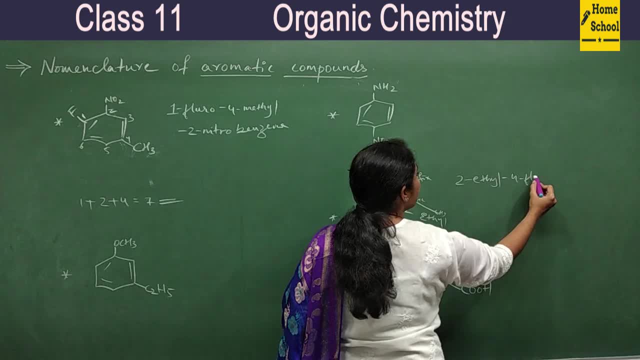 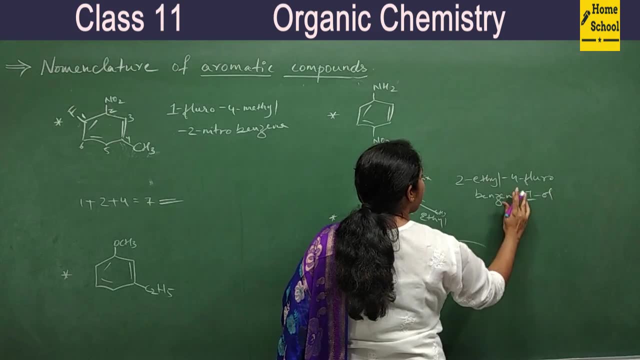 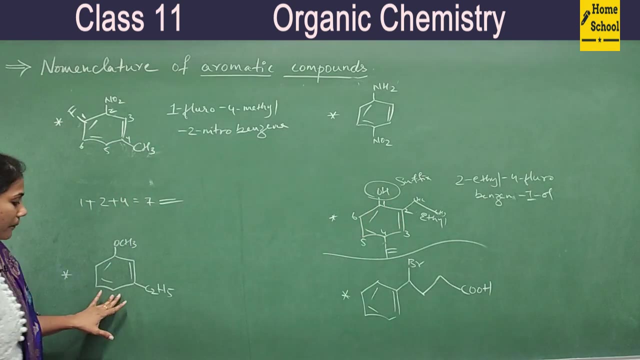 then 4-fluorofluorobenzene, benzene 1-ol. okay, So this is how we will name Clear, Fine. And now coming back to this compound, right, So here this is methoxy group and this is ethyl group, So methoxy is more. 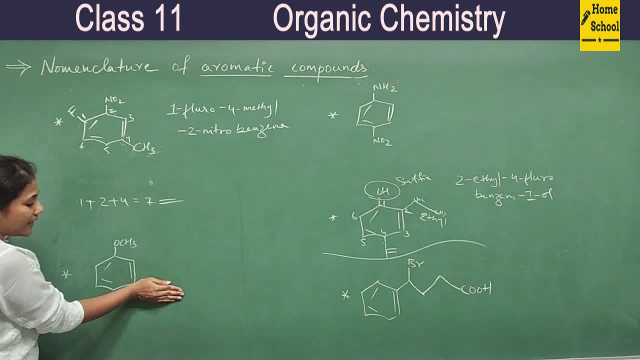 preferable. okay, You know that if I close this, this is like anisole. We know its name: anisole. that is a worldwide accepted IUPAC name. okay, So this is actually anisole. so this carbon gets 1,, this is 2,, this is 3.. I can name this as 3-ethyl, 3-ethyl-anisole. 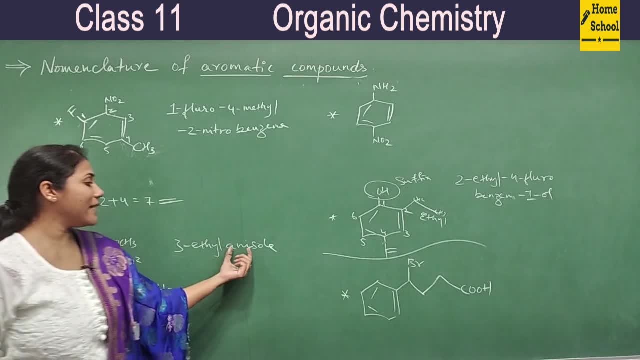 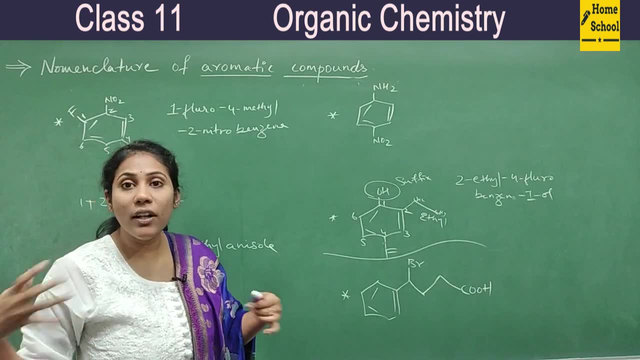 okay, So I can use the core basic name right: Anisole. So you must be familiar with phenol anisole aniline. So all these compounds are very, very important. okay, Fine, Coming to this. 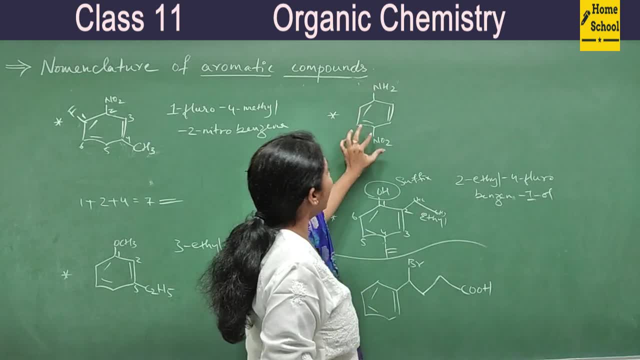 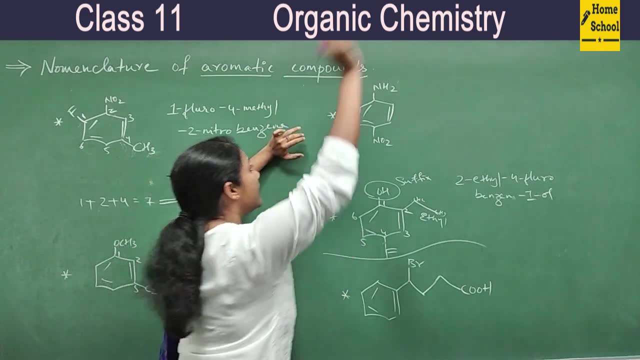 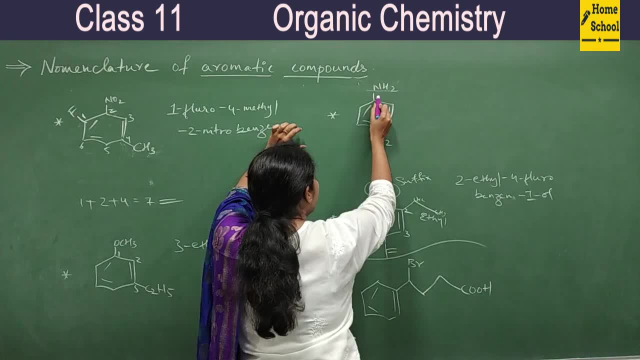 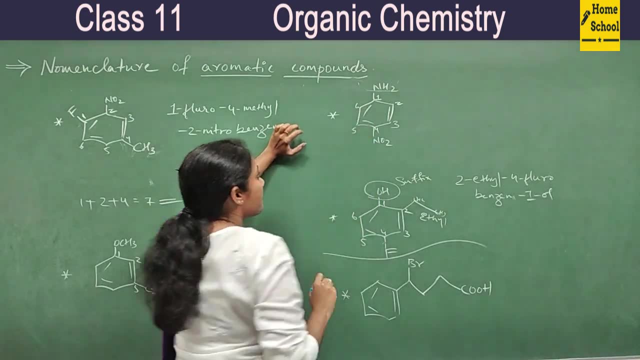 is given for amine group. So amine group, having carbon, will get number 1 position. So this is 2,, this is 3,, this is 4,, this is 5, and this is 6.. And this group's name you can write it as a: 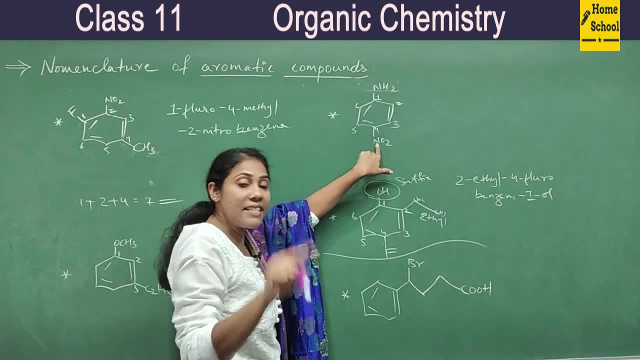 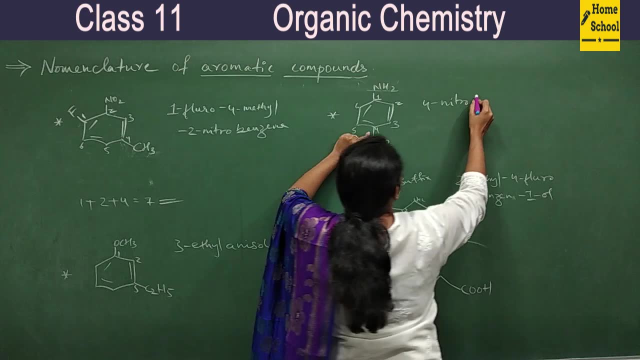 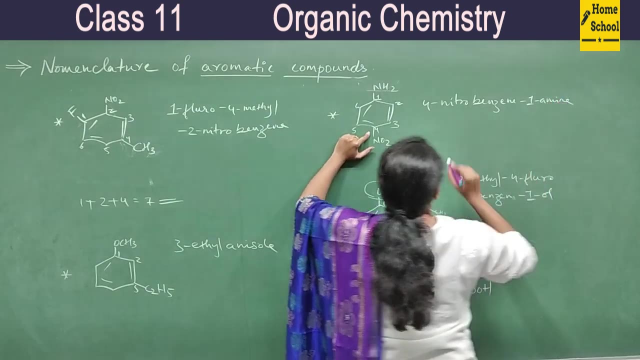 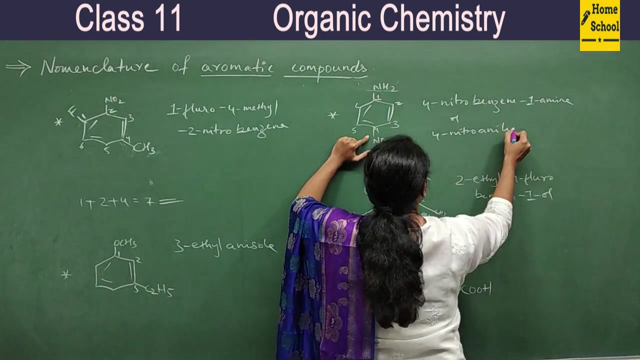 suffix, And its name. you will always write it as a prefix. okay, So I can write its name as 4-nitro-benzene-1-amine. okay, Or I can write its name as 4-nitro-aniline aniline, You know. 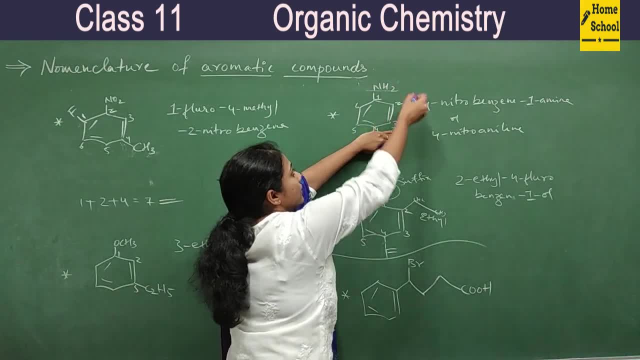 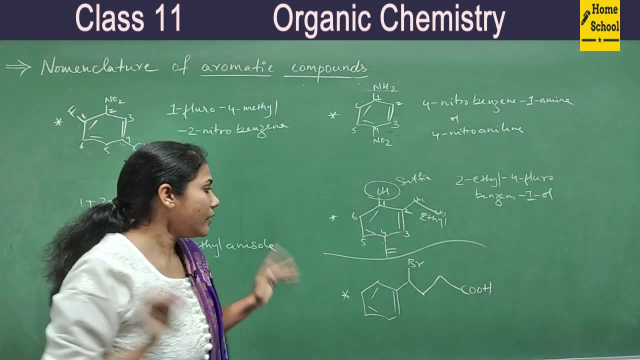 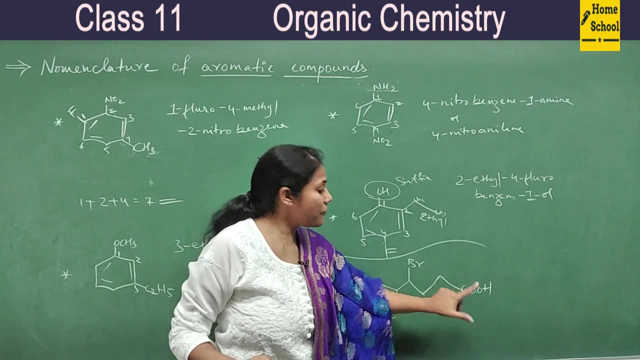 if I close this, what is this basic compound? It is aniline, So 4-nitro-aniline. This is another way of writing a name. Fine, And coming to the last example, this is a homework question for you. You have a side chain. Side chain has a functional. 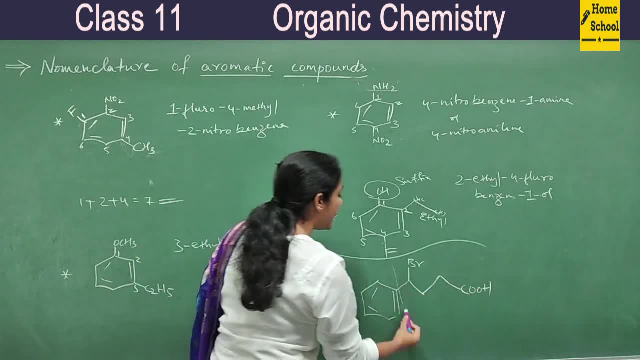 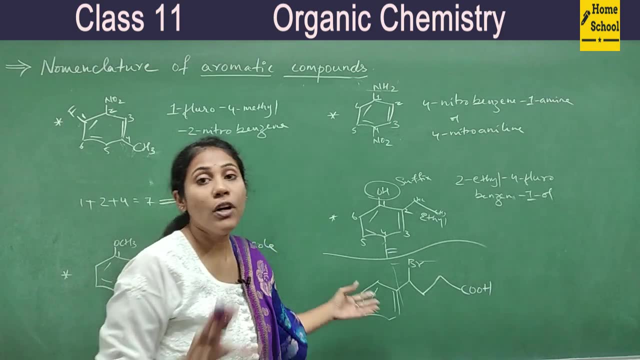 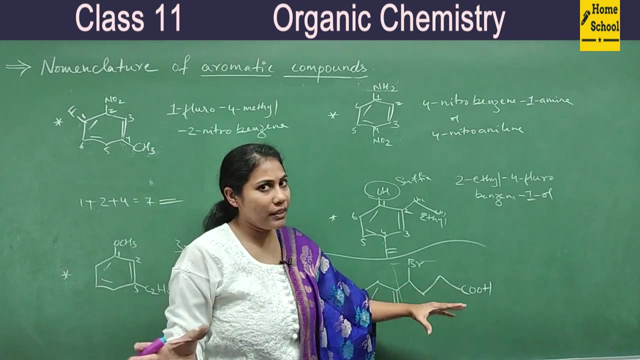 group, Then definitely you must consider this side chain as your parent chain. The name of benzene. you have to write it as a prefix. So when you have to write its name as a prefix you must use the word phenyl. So I taught you. you know naming of such compounds, right. So